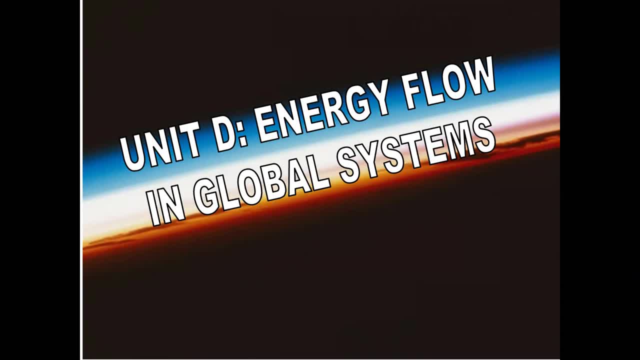 There's not a lot of like facts and things you need to memorize, so you should be good in this unit. Keep in mind that this unit does not take very long to do and it can be summed up in roughly five minutes. but we are going to be a little bit more in-depth than that and hopefully you guys have a good understanding of this unit. but just keep in mind that it's a simple unit. 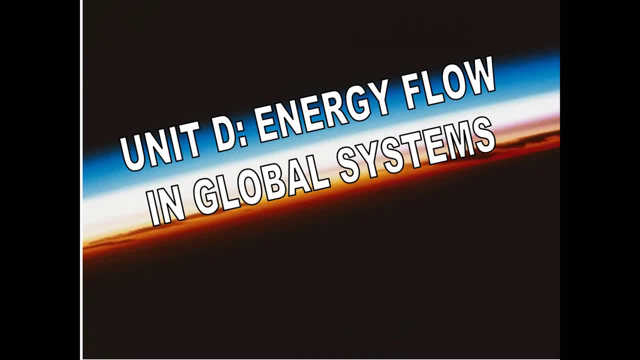 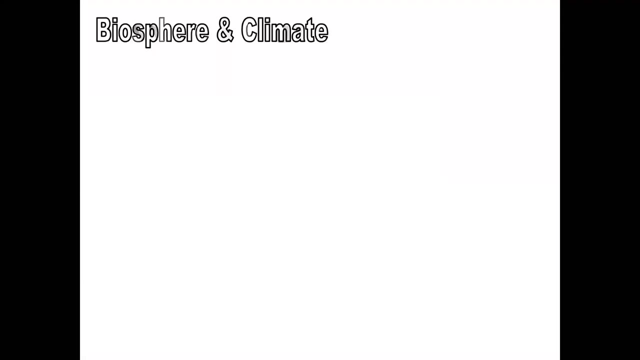 So even if we do fly by something and you're like, oh, I don't really quite get that, well, It is what it is, because it's probably not that important. Okay, so let's begin. So, biosphere and climate. so we're just going over some key terms right now. 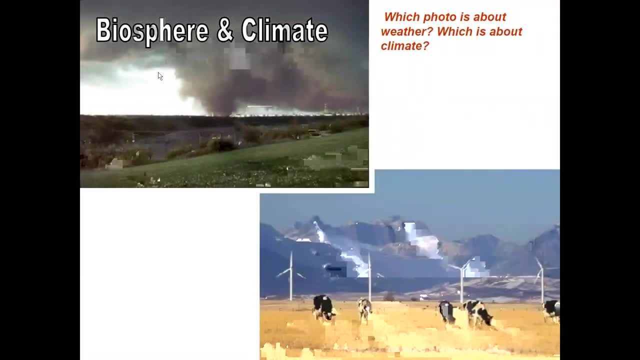 So it gives us two pictures and it asks which one is weather and which one is climate. So you would often hear someone say, oh I like the weather today, Oh, the weather's really bad today. Well, the weather can fluctuate day by day because weather is a daily type of measurement for, like, the daily temperature and conditions of where you live, but climate is an overall overbearing, like a trend in the weather that you experience. 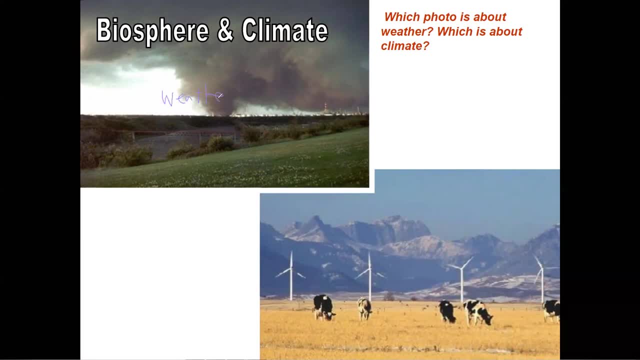 So I would say that this is weather, and I would say that this, This would be climate, because I don't think that a tornado would be an everyday type of thing. It's a fluctuation, It happens and sometimes it doesn't happen. 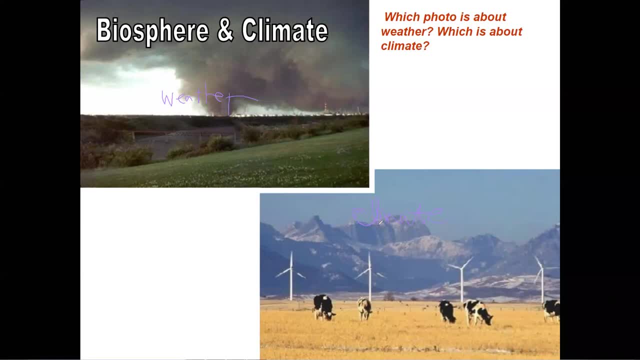 And this is like an overarching thing- Like probably in this prairie the weather's always like this. That's why you can grow like so much of this grass and stuff. So let's see if I might Mouse. 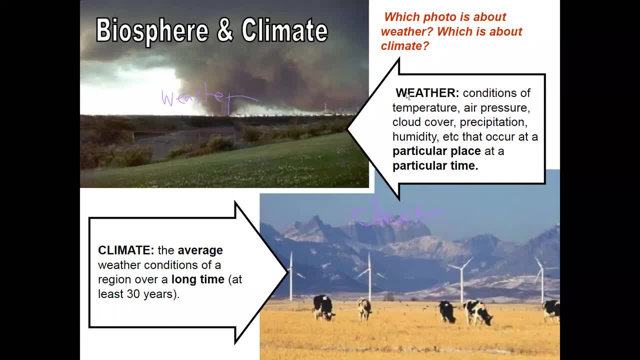 Okay, All right. So this is weather. So weather is defined as conditions of temperature, air pressure, cloud cover, precipitation and humidity. you know that occur at a particular place and a particular time. So, like I said, that's a daily occurrence type of thing and it can fluctuate a lot. 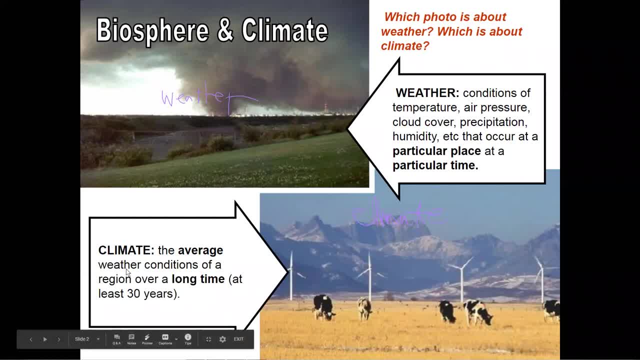 But climate is the average weather conditions over a region of area over a long time. So it's just the general idea of the weather barrier. So If we hit a snowstorm in the middle of the summer, we're not going to say that oh, the climate is really cold. 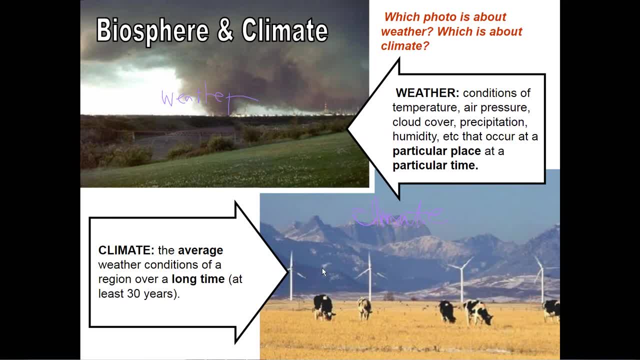 We would rather say something like: the climate is pretty hot in the summer because obviously we only get a snowstorm every day, So it's an average. So you need like evidence to support your claims on describing the climate. Let me clear my drawings. 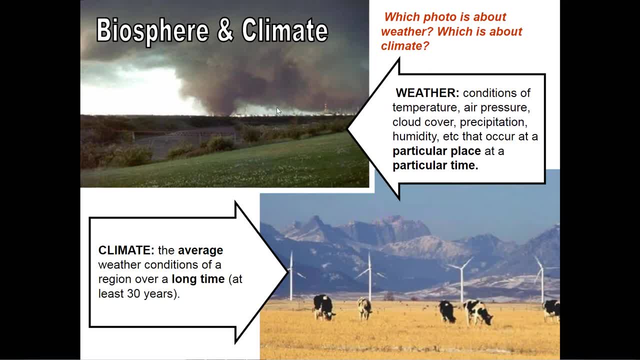 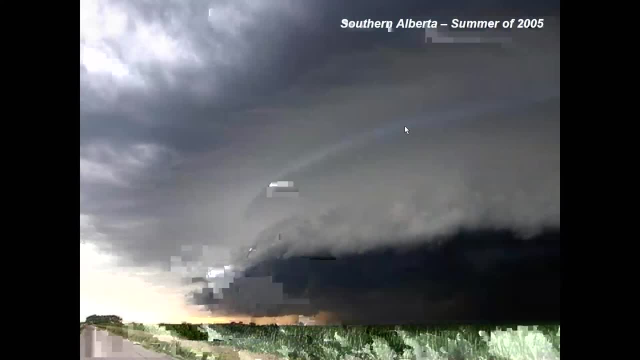 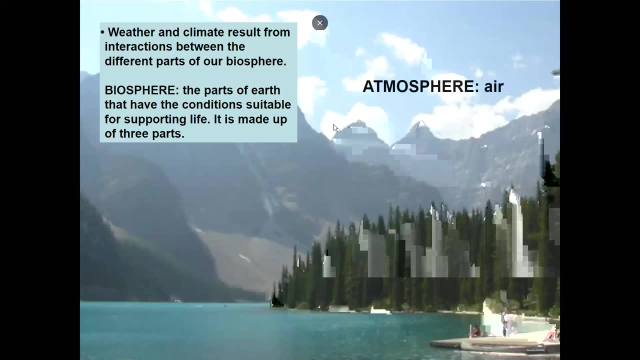 Clear my drawings. Okay, All right, So this is southern Alberta, summer of 2015.. These are just pictures, So now we're on some actual notes. Okay, So the weather and climate: right, they interact. They are interactions of different parts of the biosphere. 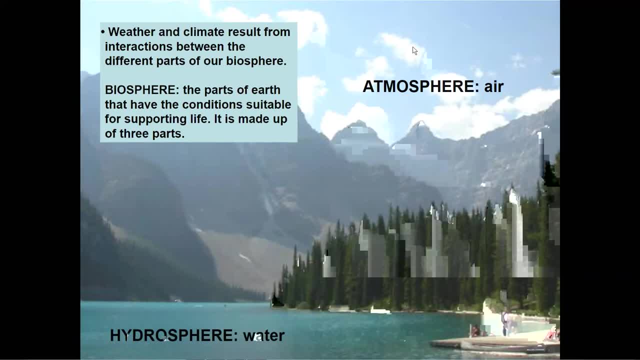 So the biosphere is just where the earth on life happens And just the nature-y aspect of it. So a more scientific term is written here: The parts of earth that have conditions suitable for supporting life. It is made up of three parts. 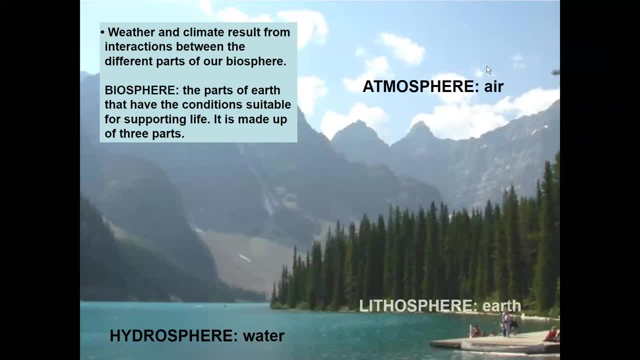 So it says two out of the three parts here. So the three parts are the air- Oh, okay, Well, I don't know how to use that- Okay, The air, the water and the earth. So atmosphere, we all know that's air. 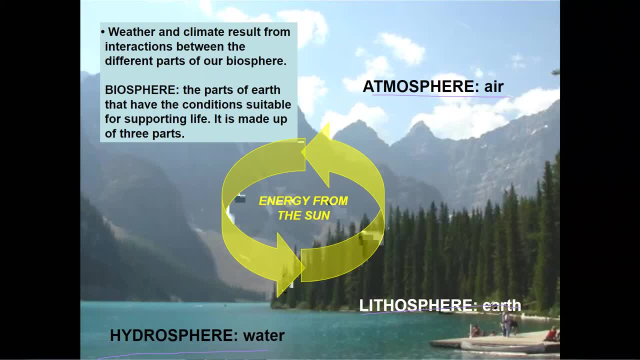 Hydro. hydro meaning water, And then lithosphere. that's just something you need to memorize, And they interact each other, all because of the energy from the sun. So the energy from the sun can help the water cycle. It gives plants and animals a place to live, a suitable habitat to live. 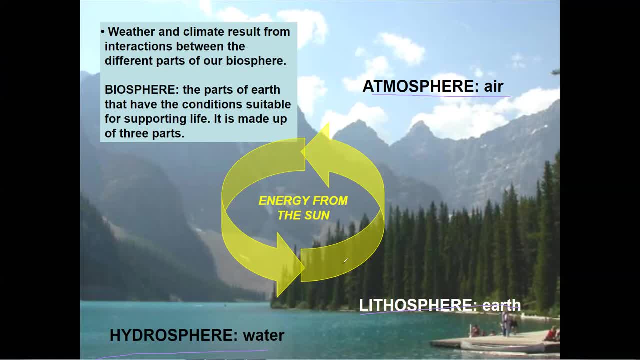 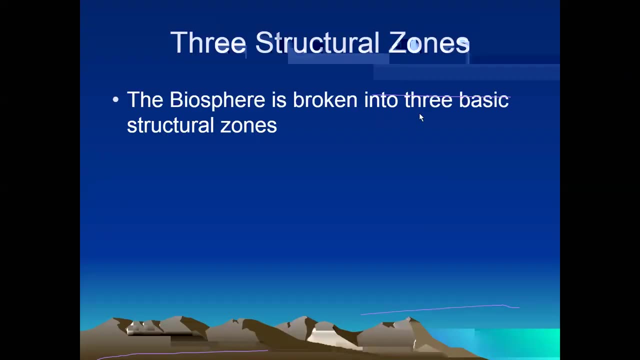 And our air can trap in the sunlight to heat the earth up. Okay, Okay, Okay, Okay, Okay, Okay, Okay, All right, So now we're going to go through the structural zones. Okay, So I believe we just went through that part. 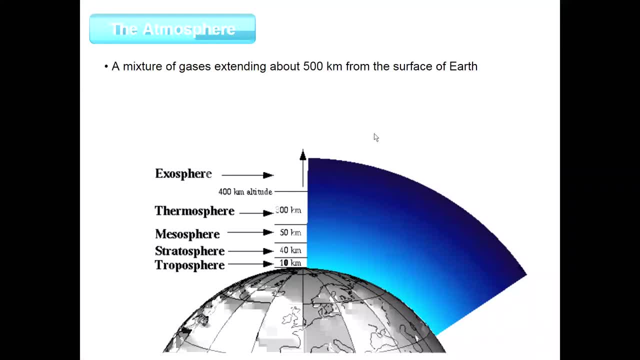 So we're good, All right. So let's go over the atmosphere in detail. All right, So the atmosphere is just air, Right, But what is air made out of? Surprisingly, it is made out of only 21% oxygen. 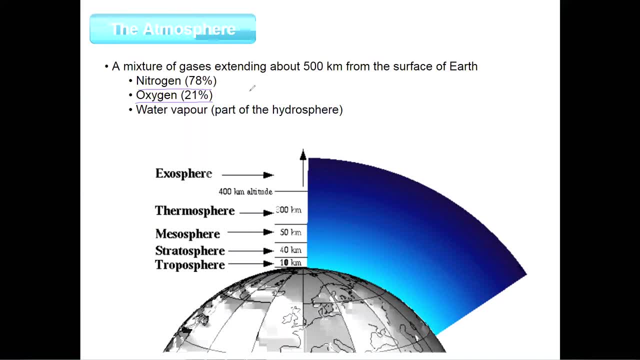 but 78, nitrogen and um. you don't even know any specific data, data like um, specific numbers for this unit, but you just need to know. you know the general trend of it, okay, and the atmosphere here is around 500 kilometers out and, if my memory is correct, i believe the first 10 kilometers is. 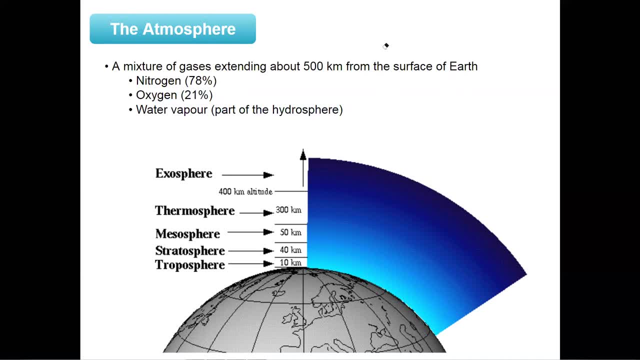 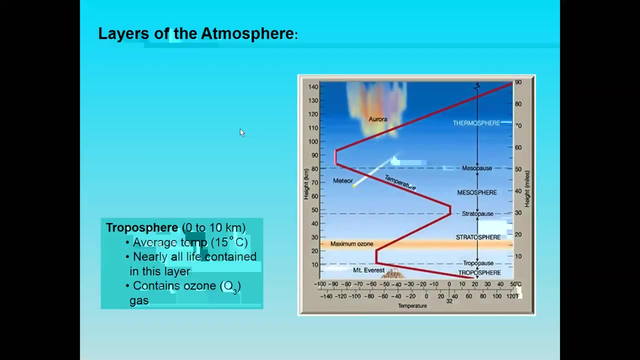 like um, where we live. so i don't know. that kind of surprises me, because 10 kilometers- you wouldn't think that's a lot, but that is the amount of air that we need to live in. okay, all right, so these are the layers. all right, so this graph is just showing the temperature and how it increases, and 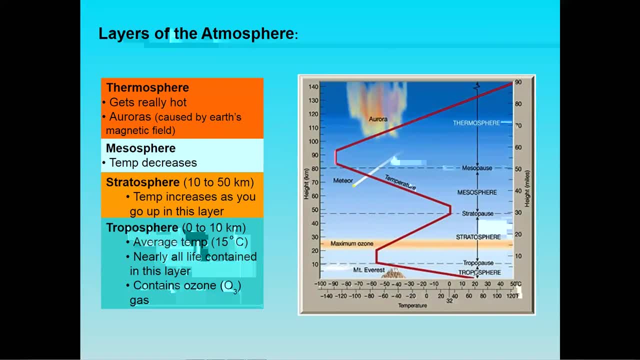 decreases per layer of atmosphere. so the way i remember it is it always goes hot, cold, hot, cold, right. but what if you don't remember whether it goes cold first or hot first? so i just think of: uh, as you go higher, right, you get colder. so i just 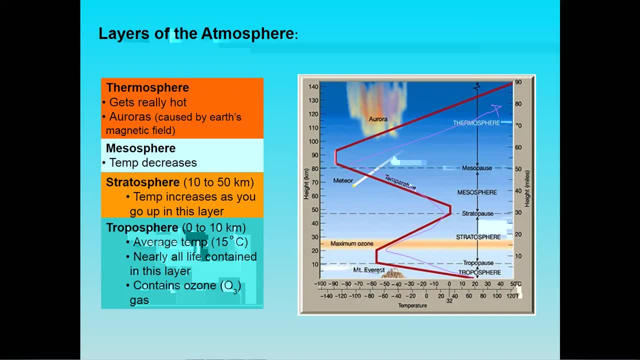 think about mount everest. i see that right here, and how on mount everest it's really cold. so that's why i know it goes from hot to cold and cold to hot and cold to hot. right, sorry, okay, so the layers are called. well, this layer is called the troposphere, the stratosphere. 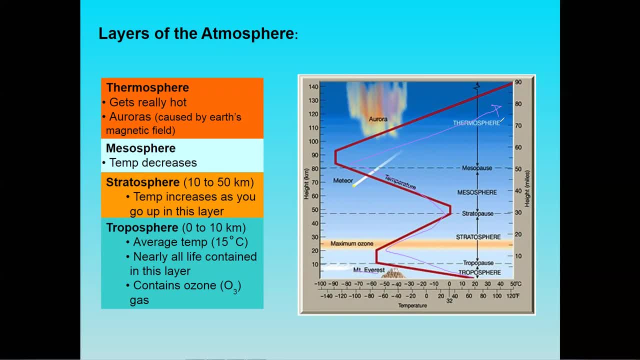 the mesosphere and the thermosphere, and it's not really important, but this is the one where we live in. this has ozone in it and ozone traps uv radiation from the sun, so it's very important to kind of know what's in there. this was a pretty irrelevant uh layer of the atmosphere, and then this is called thermosphere. 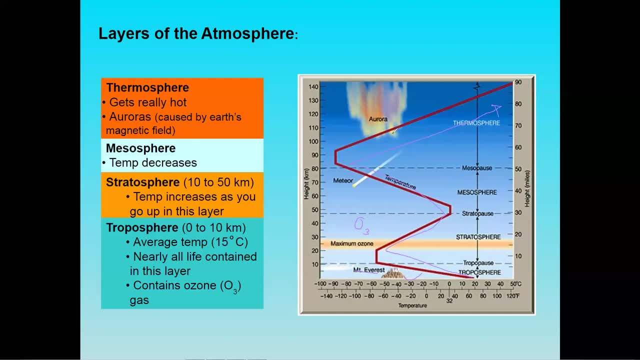 it has aurora borealis. it has aurora borealis and they're like these, like streets of light caused by, like the magnetic field interacting with the earth or something like that. like yeah, basically the unit to me is just something like that, because they give you very simple. 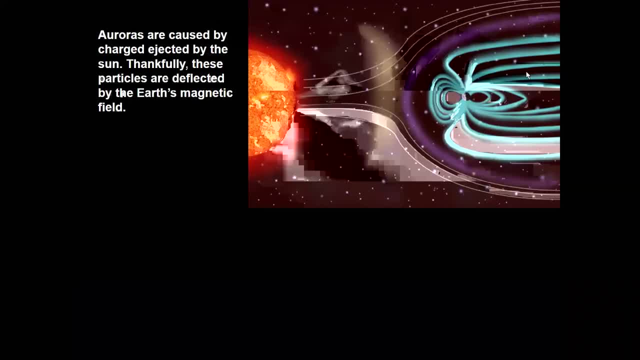 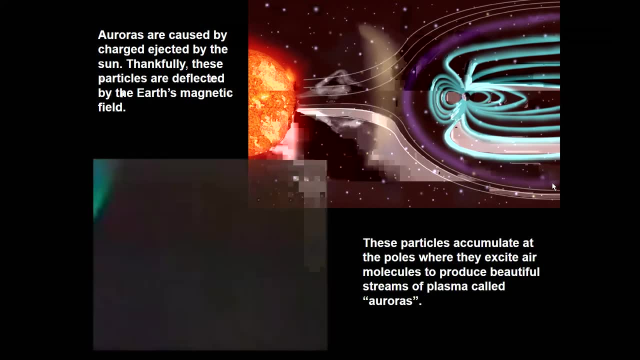 understandings of really complicated things. all right, All right. oh, look see. deflected by the Earth's magnetic field. So these particles accumulate at the poles where they excite air molecules to produce beautiful streams of plasma: polar aurora. Okay, see the definition that they gave us. 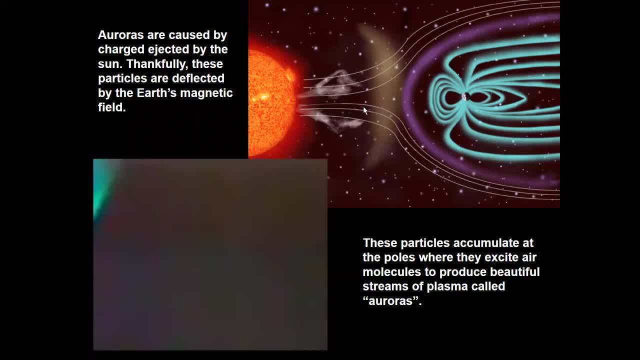 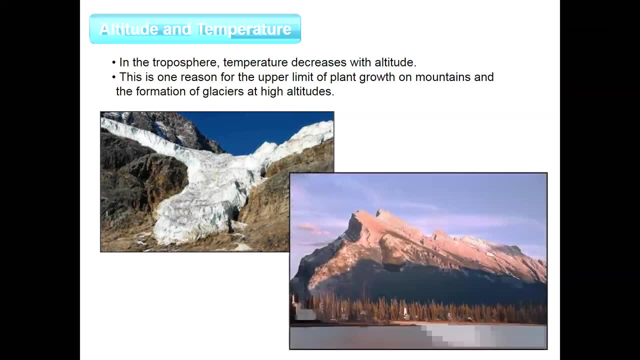 was pretty standard, not very helpful, but just deal with it All right. altitude and temperature: Okay so altitude is how high? something is right, So as your altitude in our troposphere, right in the place that we can survive in. 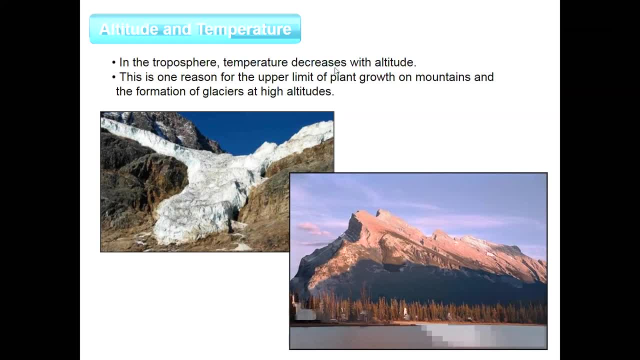 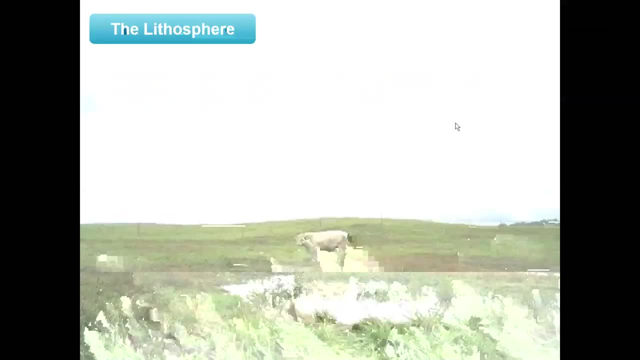 as the altitude increases, right, the temperature decreases, All right. that is why there's snow on mountains and why it is really hard to breathe, because there's not a lot of air. Okay, so Earth's temperature, Earth's atmosphere, All right. I don't know why it said Earth's atmosphere. 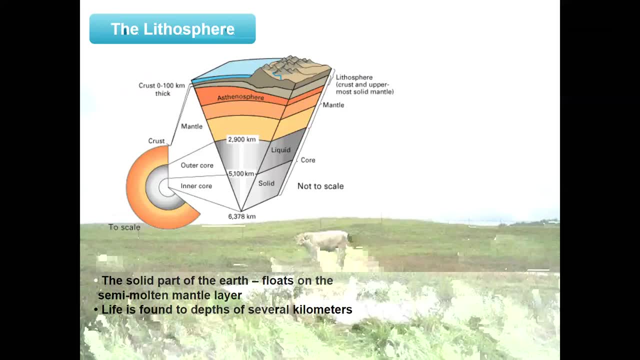 I know the next slide. I don't know why it was lithosphere. All right, so lithosphere is our Earth and obviously there's, like the actual Earth, Earth like dirt terrain and water, and under that is all the lava right. 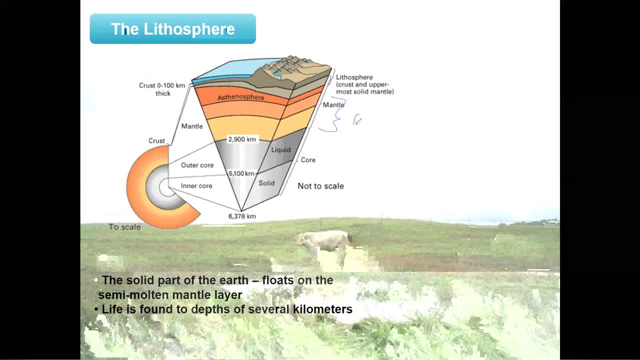 You don't even know all these terms and stuff, but lava, Earth, and then beneath that is the Earth's core, which is like metal or something. So just like, just know that it's core. It goes from hard to soft, essentially okay. 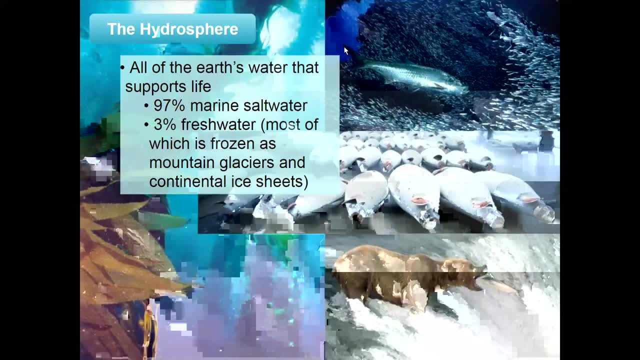 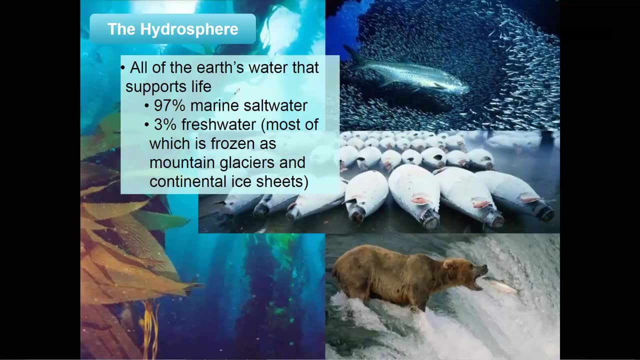 Why? All right? hydrosphere, All right. so the ocean is the hydrosphere, And all of Earth's life depend on water to some extent, because we need it in our body and we need it to grow. It's your body. 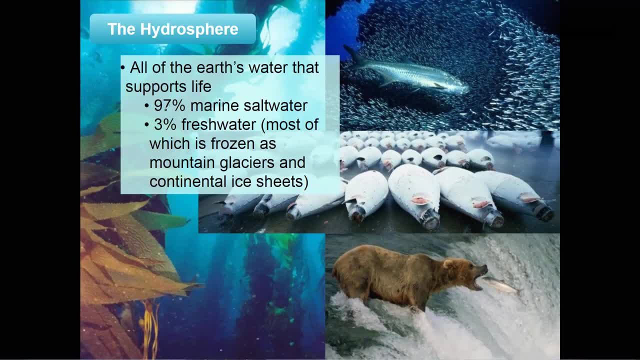 body utilizes water- and water okay, and 97 of it is salt water. three percent is fresh water. most of it is frozen as mountain glaciers and continental ice sheets. so this basically means is that, like um, we should be watching out for our water consumption, because we don't have a lot. 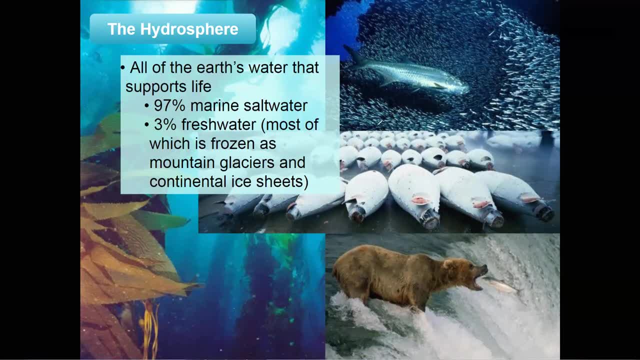 water to use and we have to go through a lot of processes like filtering them and whatnot, and requires a lot of technology, money and resources. so it's best to conserve water, just in case in the future where we don't have any fresh water left and we have to do all of these things. 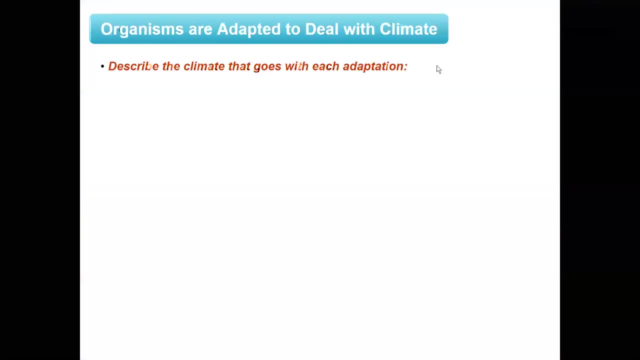 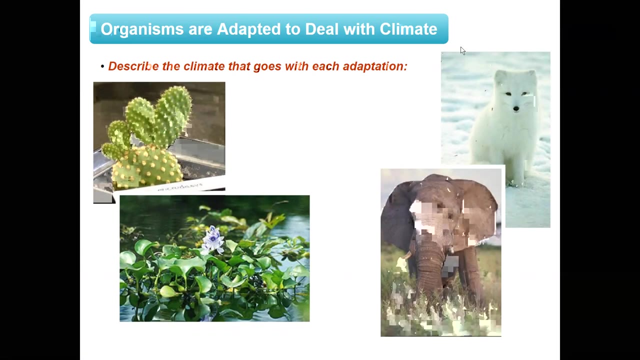 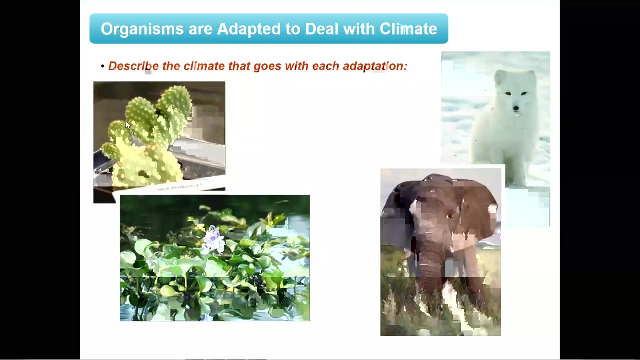 all right. so adaptations, right. adaptations are changes that animals or the organisms make to respond to stimuli in order for them to survive in a situation. so a cactus, a lily or something, a fox and a elephant. okay, so describe the climate that goes with each adaptation. so i believe. 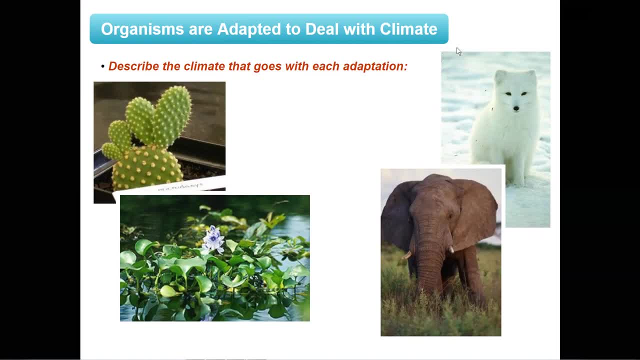 the fox lives in a cold climate, so therefore, if it's cold, it needs something to keep it warm, so that's why it has fur. okay, the elephant lives in a very hot climate in africa and it has big ears, so these ears can act as fans, or it can it? 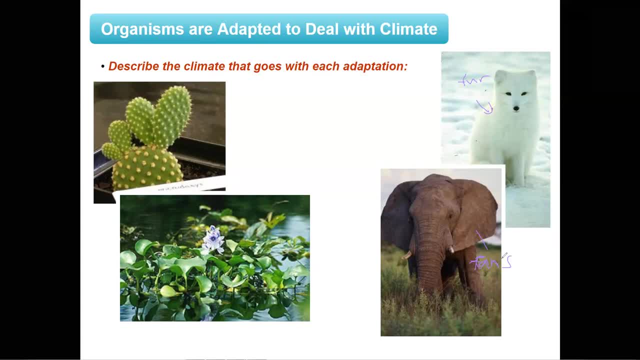 you volume? did you touch on um surface area to volume ratio and bio? hello, yes, okay, yes, so the surface area to volume ratio of the elephant ears allows the heat to be, um, like taken out very easily, like diffused very easily, very efficient. and then the and the cactus lives in a dry climate, so it will, so it, so its leaves are flat. 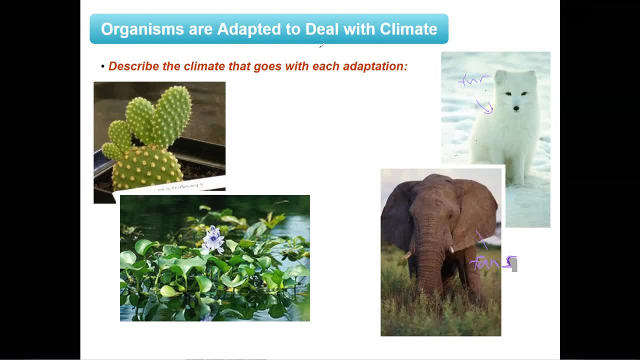 because once again there's a lot of heat, so let's go. okay. so fat leaves prevent water loss. interesting. so it was in a wet climate, so air filled bladders for flotation. okay, this was a pretty bad picture. i don't know why they put it there. all right, large, thin ears, maximize heat. 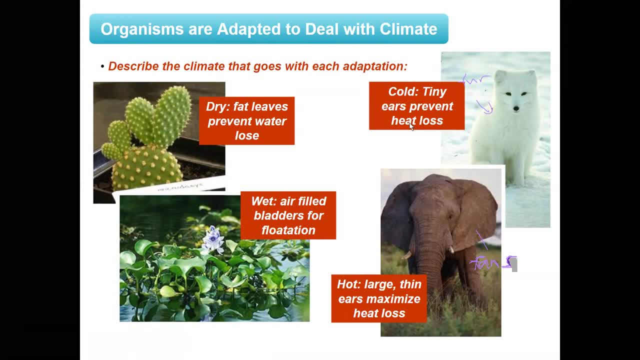 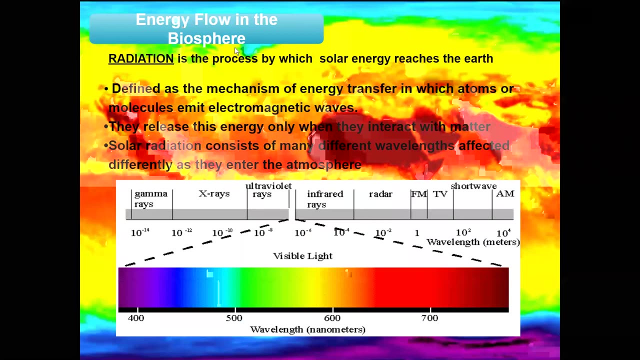 loss. okay, then cold tiny ears prevent heat loss. tiny ears, what is? okay? um, very interesting, but uh, yeah, let's just move on. but uh, yes, okay. so radiation, all right. new term defined as the process by which solar energy reach solar energy reaches the earth, right? so, oh my god, why does it? 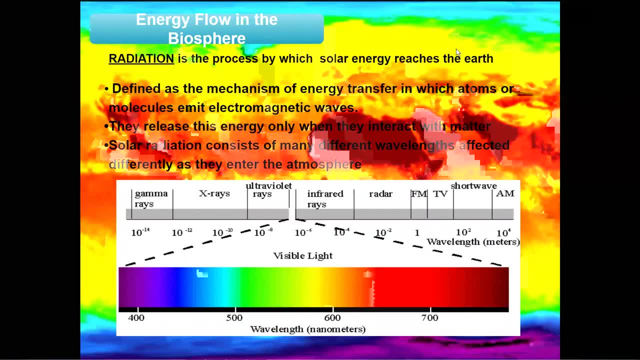 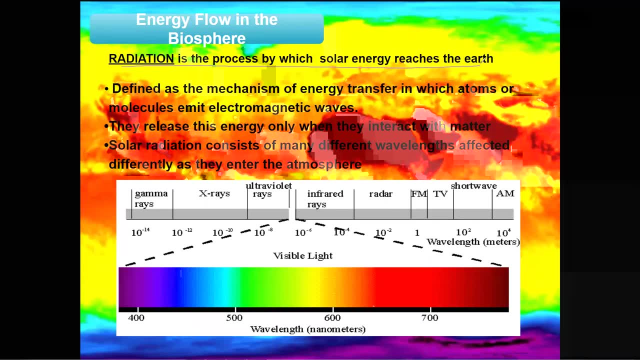 go in there. okay, all right. so in simpler terms, it just means um the light that comes from the sun, like that's it re-radiation, and then this radiation can can be of different wavelengths of light, and these wavelengths do different things, like ultraviolet rays are, like all uv light. right, that is uh that. 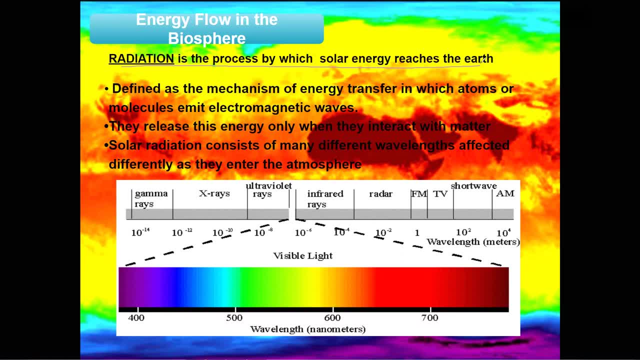 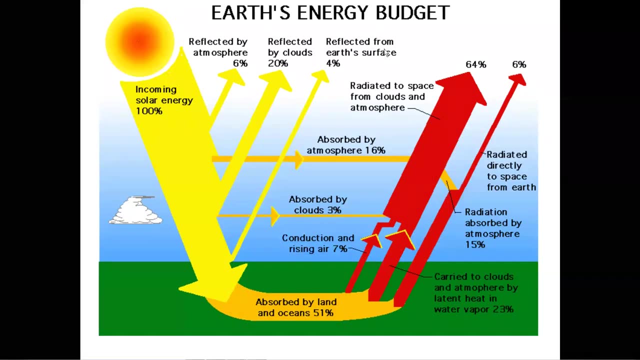 can mess up your skin and all this stuff and infrared things like that. okay, let me do the next one, all right, so this is just a quick diagram showing you what happens when sun, from the light, reaches earth, and i really hate this diagram when i was looking at it because it was really confusing and 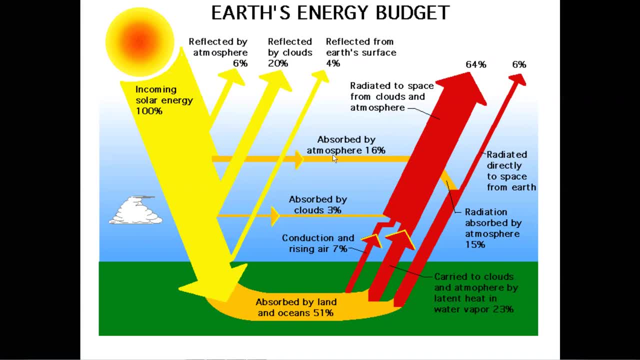 the percentage never added up, but, um, i believe it's 19. so, if i remember correctly, like when i finally understood it, oh my god, this. i think this meant what is happening. okay, this meant that we wouldn't be able to have the light that would be in a more. 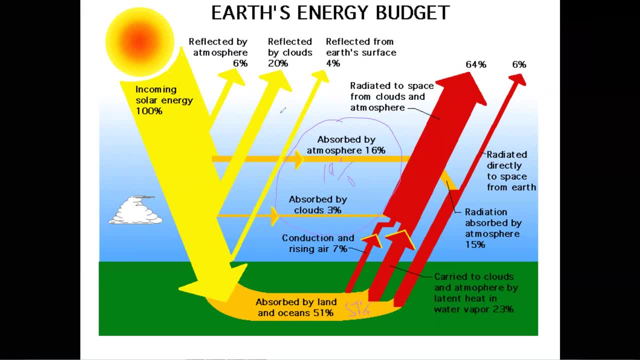 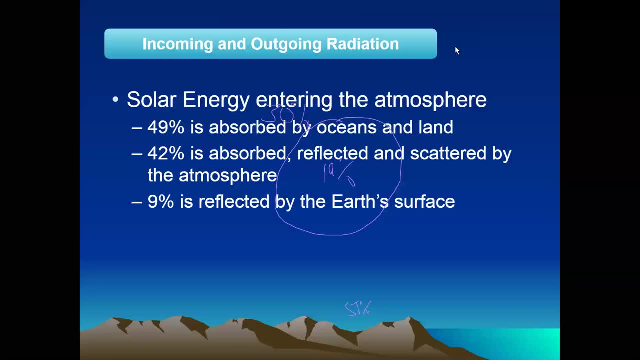 luminous light from the sun. when the sun reaches the earth, it's not just to some very tiny doll per se, right? it's just something that's gone to a big space and it's lost. we're not going to put it in our electronic application, right? so i'm trying to understand why, as a 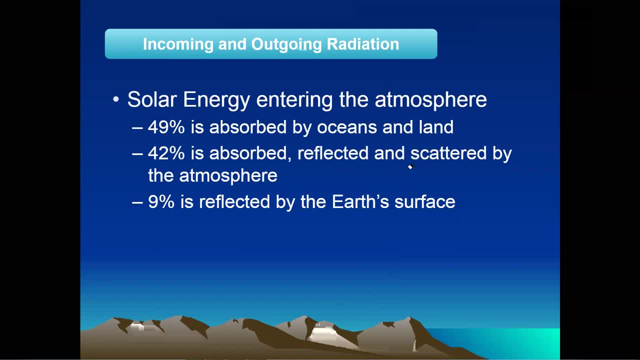 think sometimes the ability to get the light that we need, we need from the sun, to actually capture it. oh my god, wow, that's so cool. all right, so this is the same thing, like as we're just showing you. uh, the perception is different, for for what the last, for what the last thing said? 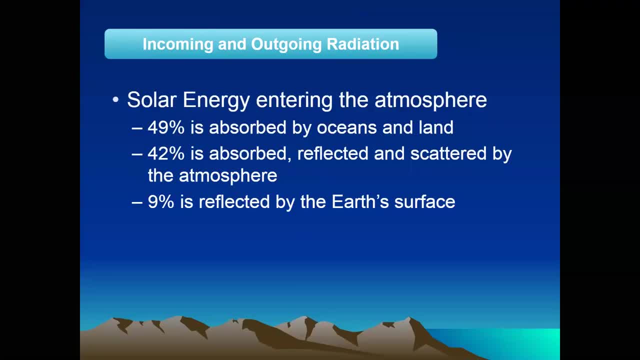 Sorry, what the from what the last thing said, so I don't know which one to go by, but honestly I would probably go by this set of data. this set of data because a teacher made this, so they probably have a good understanding. 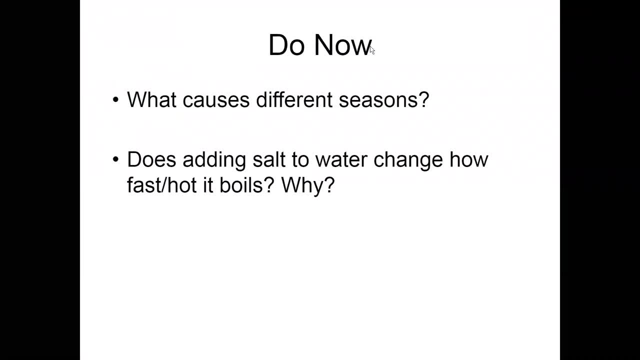 of what's happening. Okay, what causes different seasons? All right, well, to put it in simpler terms, the earth tilts on the axis and it leans toward the sun at different angles. So, if it's so, if you live on this part of the earth, 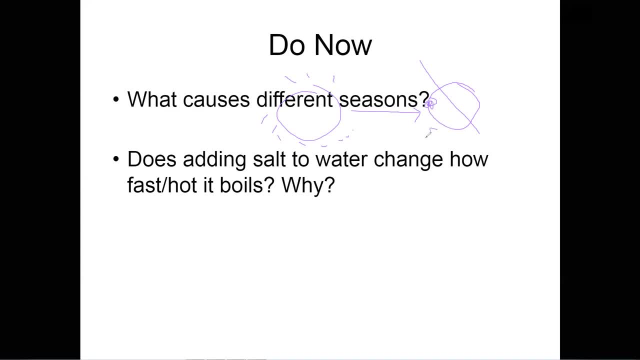 and the sun's pointing here. well, it's gonna be hotter, so it's gonna be summer, And then, if you, and if you are living on this side of the earth, right, it will be winter for you, because you are not closer to the sun. 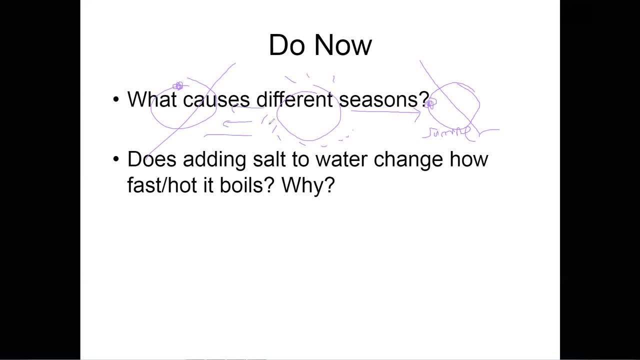 So you are not getting the same heat that you get from the sun. So that's a pretty simple way, And what determines is it is: how is that? the earth rotates in a circle- different positions, but, however, it also rotates on its own axis. 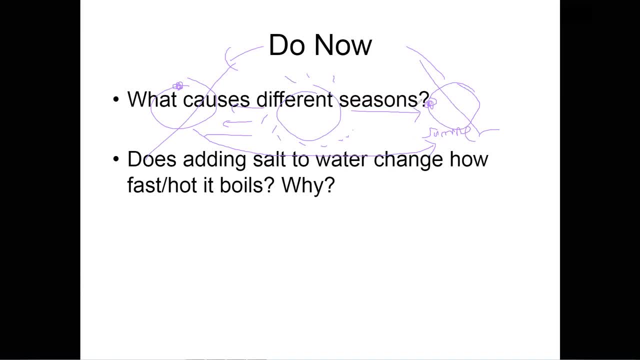 So that's why you either end up on here or on here: Yes, okay. so now what? does adding salt to water change how fast it boils? So I don't ever remember doing this question, but I believe salt does speed up how fast. 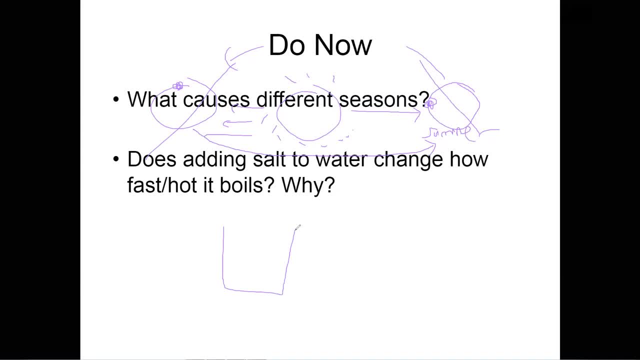 it does speed up when you add water, And the reason why it adds up is because why does it add up? I'm pretty sure it has something to do with the fact that the salt is attracted. the salt is attracted to the water and it traps it in. 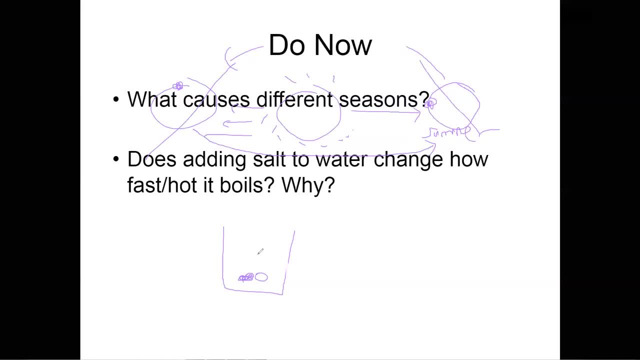 So then it's easier for it to boil. But yeah, I searched it up and it just said that: so, yay, Okay, So that's the term for that. So I think that's. let me erase my pictures. Oh, more pictures. 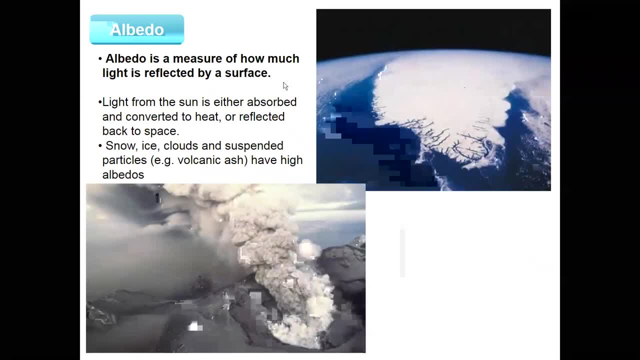 Okay, So now we have the term for albedo. Albedo is how much light is reflected by a surface, right? So things that are white, they reflect light, and they reflect light more. and then things that are black, they absorb light. 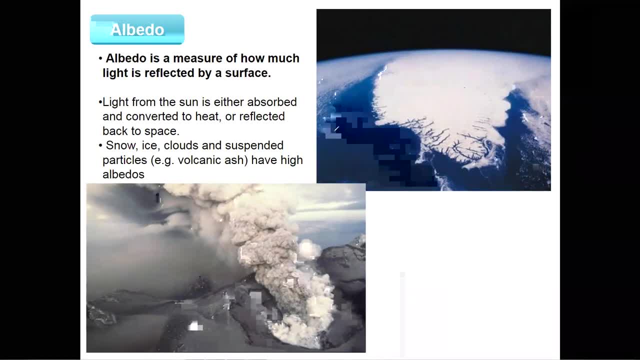 versus the black chair. in the summer you can feel the different, different uh temperature. so for here this will have high albedo because it's white and for this it will have low albedo because it is dark. pretty, pretty interesting concept, okay. so when light is reflected back to the space, it can. 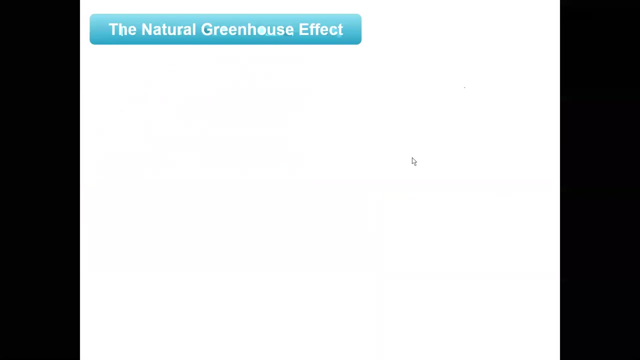 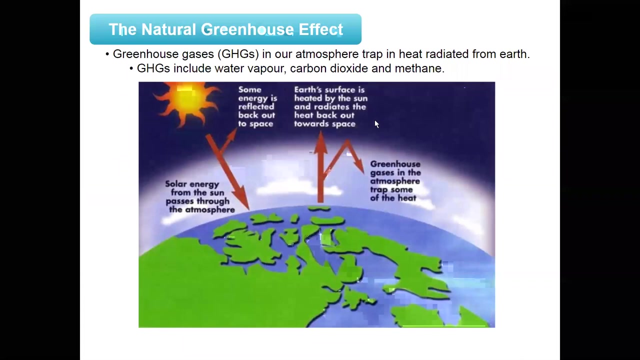 have global cooling effect because you are not absorbing the light, correct, okay? natural greenhouse effect, okay, so you've probably heard of the greenhouse effect thing. and because you're saying that it's due to doable and greenhouse gases cause global warming, right, right, um, i'm not sure i'm distracted by something, but, um, yeah, so the way it works is like you have the. 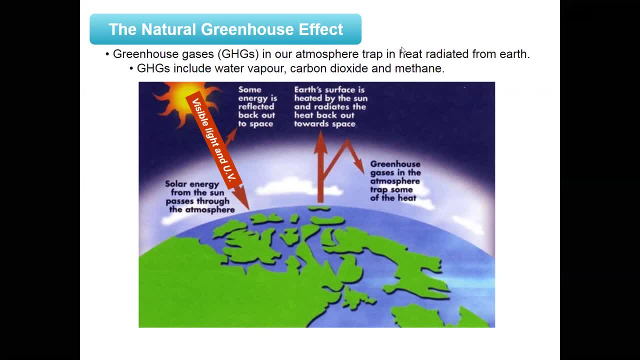 sun comes in, and then there are certain greenhouse gases that like specific chemicals and they just trap the sunlight. so then it gets really, really hot because now there's more sun, right, and that's basically what this picture is saying. okay, infrared, without greenhouse effect, the earth would be completely covered with ice. this is also true. 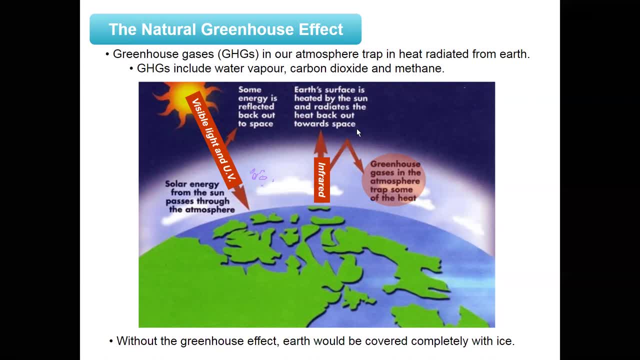 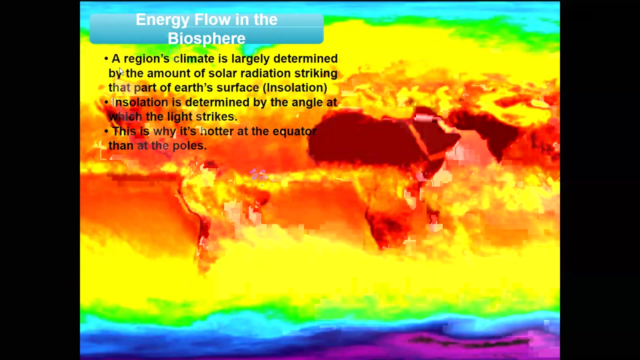 with you need a certain amount of heat to sustain life. all right, all right. oh wait, wait, something came up. my bad. okay, let's move on. okay, so our region's climate is determined by how much sun hits it. right and at the equator, the, the like, so, equator, so like, african, south american countries, rainforest. 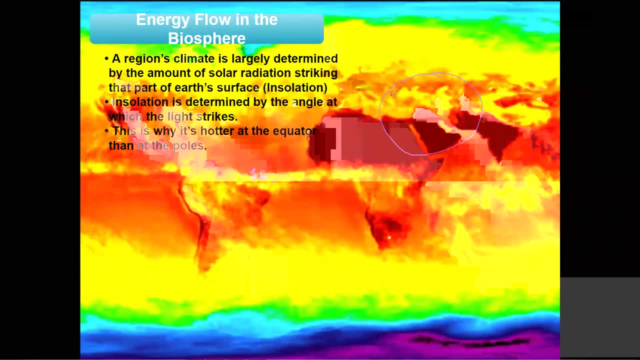 uh, there is. it is hotter because the more light hits it. so if we look at a sphere right, we can see that it narrows out from the top towards the bottom, so the light hits it. so more light will hit it here than compared to here, because it is wider and it is closer. okay. 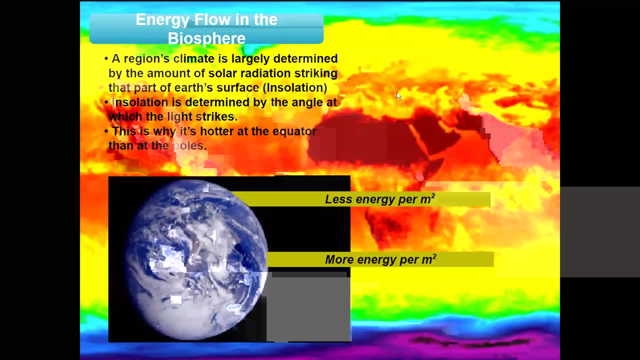 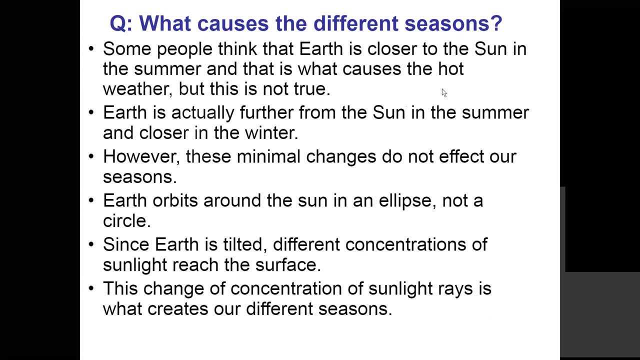 yeah, so what causes different seasons? okay, so some people think that earth is closer to the sun in the summer, but but winter. but that's not true, right? um, it's just because of the tilt. so it says that. second last sentence: since earth is tilted at different concentrations, sunlight reaches the surface and that is why our seasons are different. 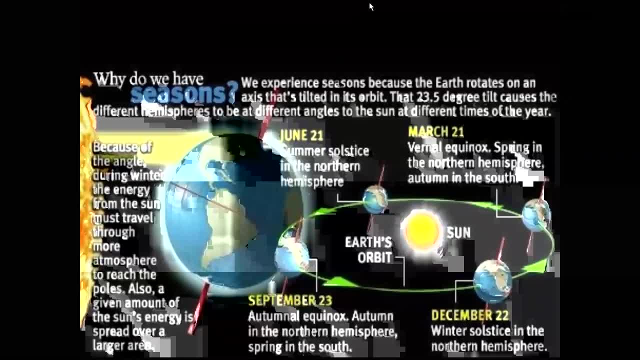 um, so let's look at this, for example. um, we're looking at this perspective, by the way. so these little, this land, all right. so from here to here, it's close to the Sun, facing the Sun. therefore, it is summer. from here it is not. it is on the. 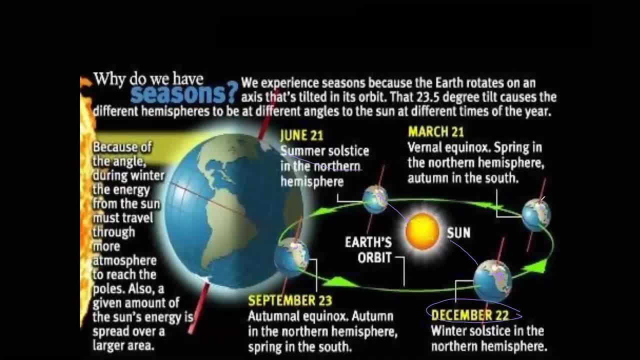 opposite side. so this is winter and then it shows you here because it's half and half, but you see how it's kind of split apart. that's that's called a equinox. so an equinox is when you have equal hours of sunlight and darkness per day- 12- and 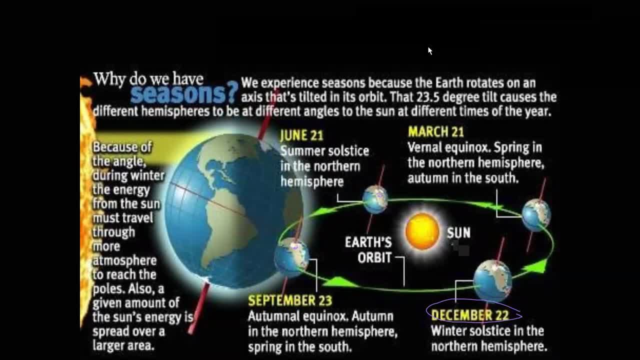 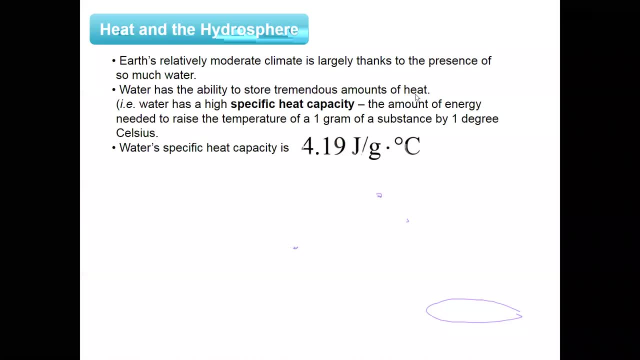 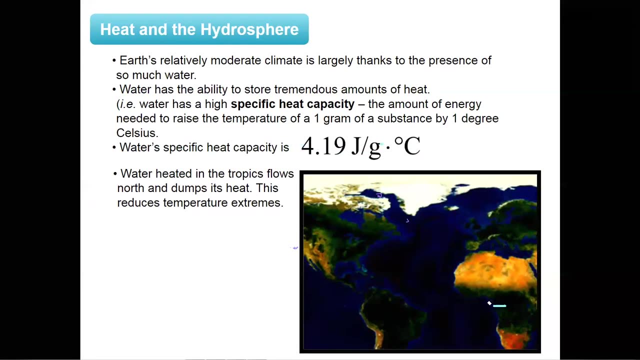 12 hours that let's get. okay, we went over that. all right. heat and the hydrosphere: all right. so why are we so good at preserving on climate on earth? well, we have a lot. we have water and that surrounds the earth- okay. so, for example, 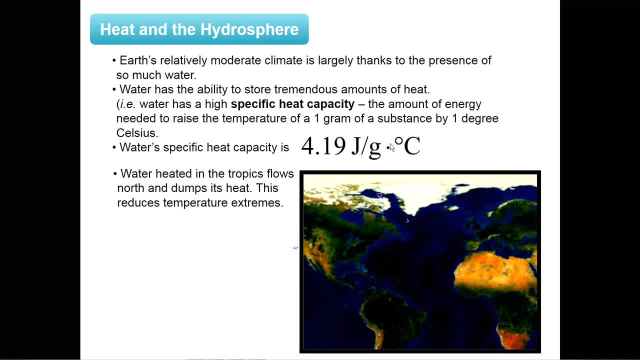 so, for example, water can store a lot of heat because it has a specific heat, a high specific heat capacity. so what this means is that it worked so like we ever. it means that it needs more energy, so more jewels, to heat one gram of something of this thing we're talking about by one degree. 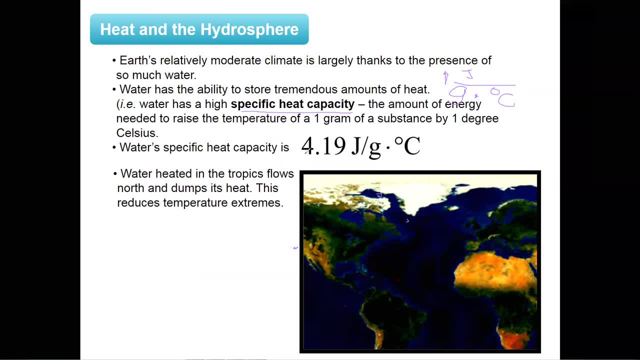 Celsius joules per degree Celsius water. so a specific heat capacity is four point one nine. I think this is the no, this is a yeah, this is the regular value. if you're an IB, you use four point one eight. okay, I don't know why, but because 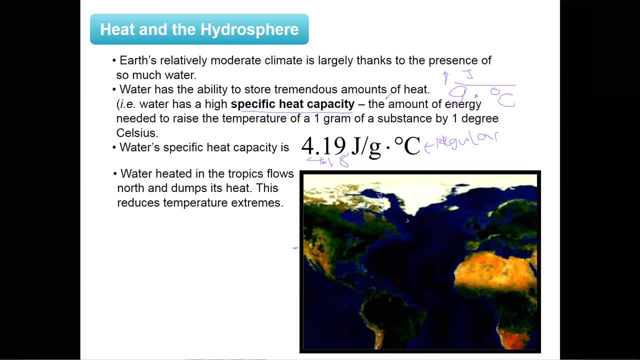 it has. it needs so much because I take so much energy to to heat it up. you, you aren't really able to like, I believe, heat up the earth that fast and the water helps keep a lot of energy in it. right, right, okay. And because there is a high specific heat of potacity, we can absorb more water in. right, because it takes a lot of energy to heat it. 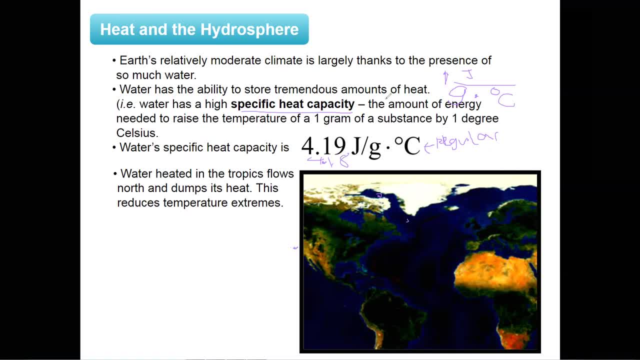 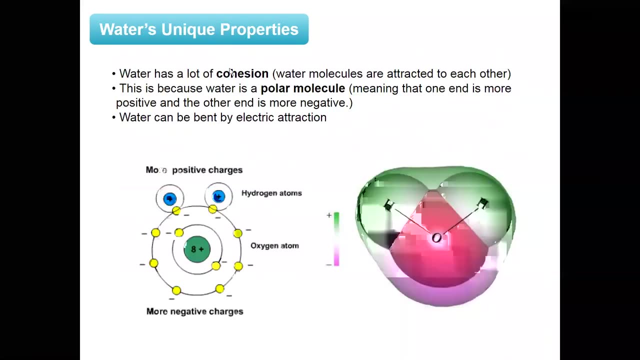 So we can actually take in a lot of energy before it being too hot. All right, All right. so water: let's just go over some water-unique properties, because we love water and we learn about it in every subject except for physics. 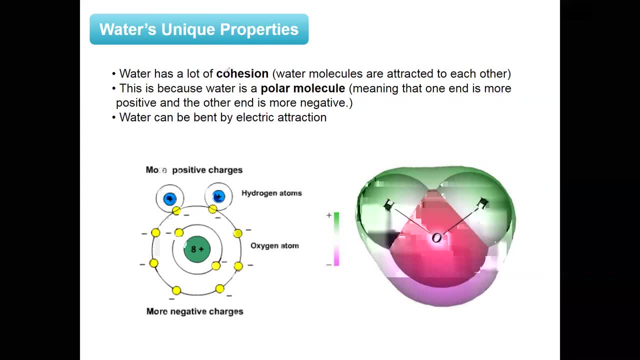 Okay, So water has a lot of cohesion, So water molecules are attracted to each other. This is because of a chemical property Where the polarity, so one end, is more positive than the other end. So something has a positive side and negative side. 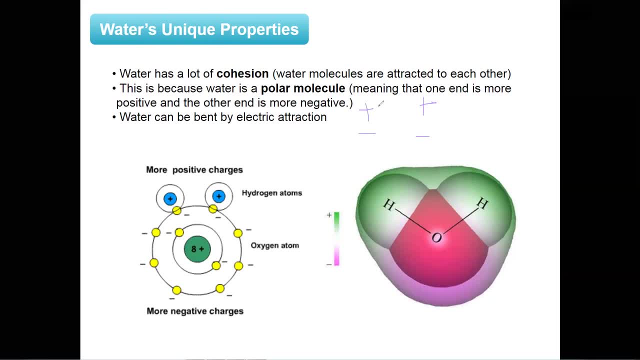 So this means that other molecules, that other water also has positive and negative side. So this positive is attracted to this negative and this negative is attracted to this positive and like there's a lot. So it goes this bad drawing, but you get the point right. 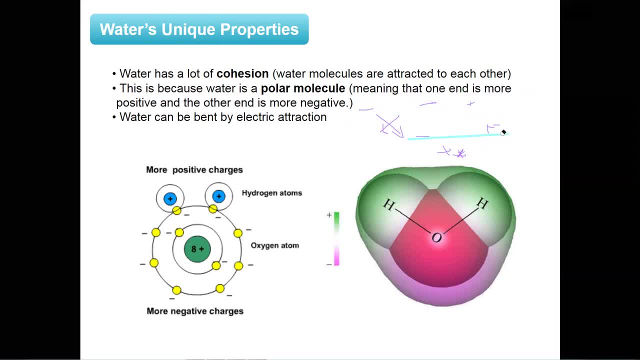 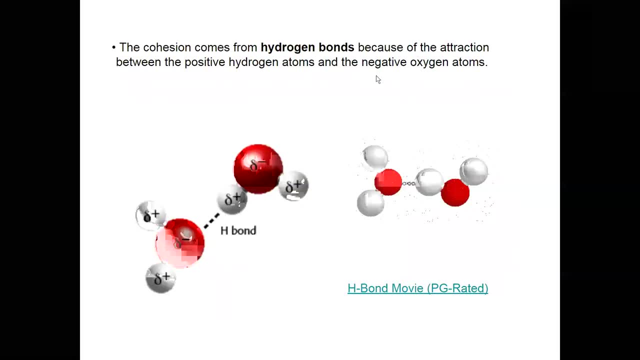 That's just a unique property, I guess, But in chemistry You'll learn more about this and it's actually a pretty interesting topic in my opinion. So water, so the cohesion, comes from the hydrogen bonds, because of the, because of the- oh my God, hold on. 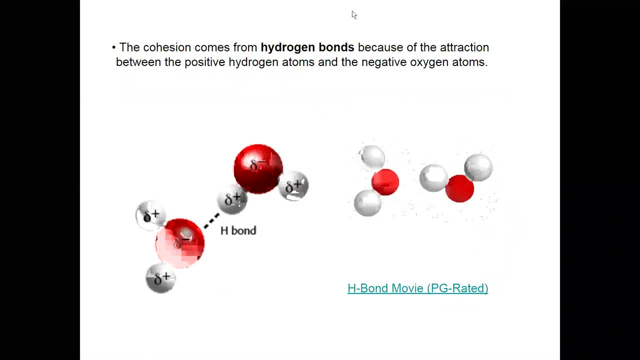 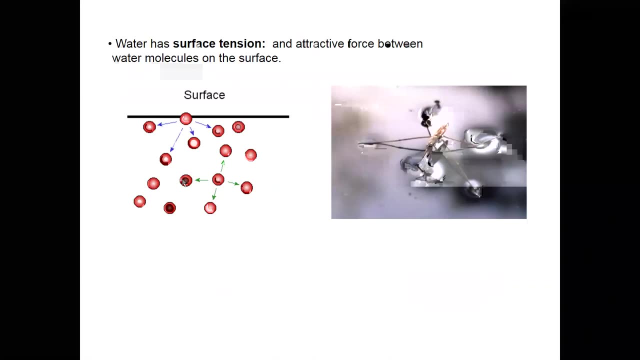 Cohesion comes from hydrogen bonds because of the attraction between the positive hydrogen atoms and the negative oxygen atoms. So one positive side, one negative side. Yes, this is positive, This is negative. Good, This is a good picture, okay. So water has surface tension, an attractive force between molecules on the surface. 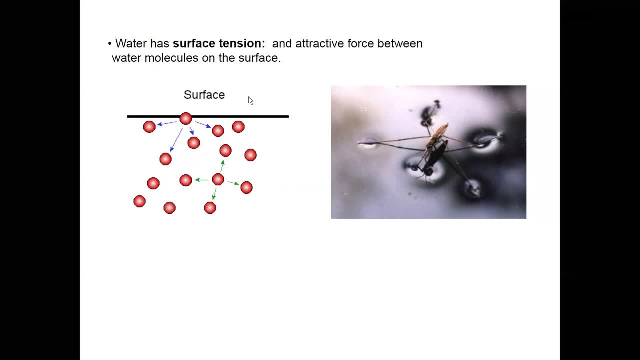 This is an also property. If you ever put a, if you ever put like, what is it called? If you ever put a water on a coin, it will form like a little like ball on top because of the surface tension. 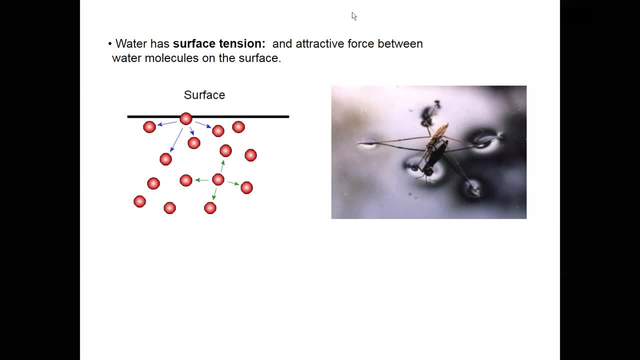 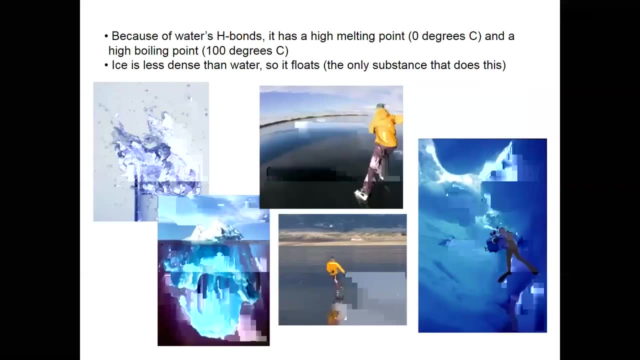 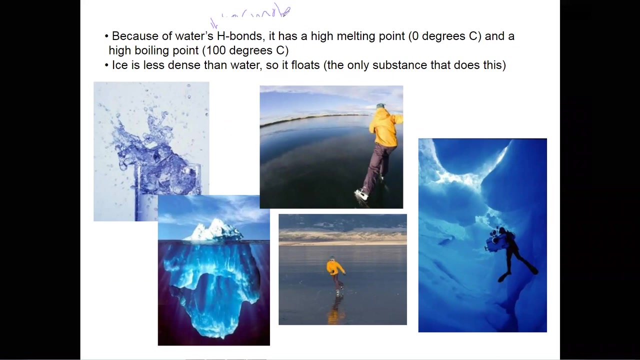 And most other things would probably just like spill or something, but water is a different breed. But I mean Right. So this is what the Celsius scale was based on on: when water turns into a gas and water turns into a solid. 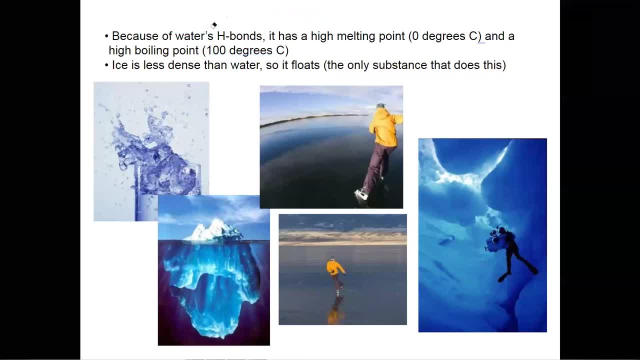 And water. ice is less dense than water, right? Remember what density is. Density is mass over volume, So that's why it floats. that's why ice floats on water, And this is the only substance that does this, And it's very important that it does do this, or else the life on Earth could most likely not be sustainable. 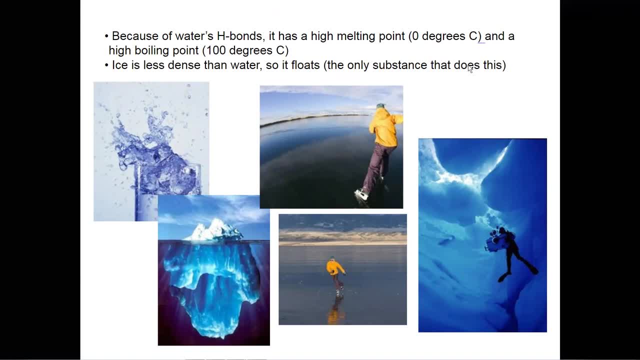 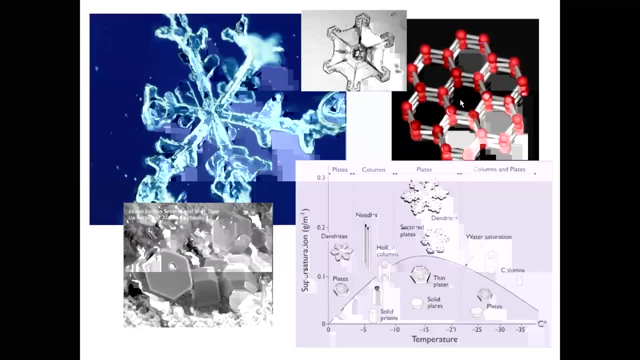 Because if the water were to just freeze and sink, we'll just get a lot of ice instead of water, right? So let's go over this. And also, in the chemical structure of ice is that there is four waters bonded together, So I believe this is ice. 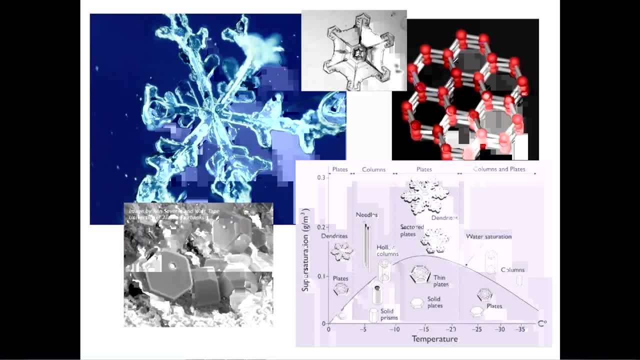 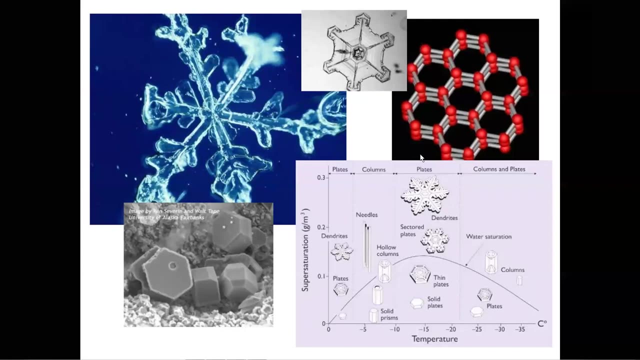 One, two, three, four, Yeah, four waters bonded together. But in liquid water there's six waters bonded to one another. So because four is more spaced out than six, it's less dense, so it can float on water. 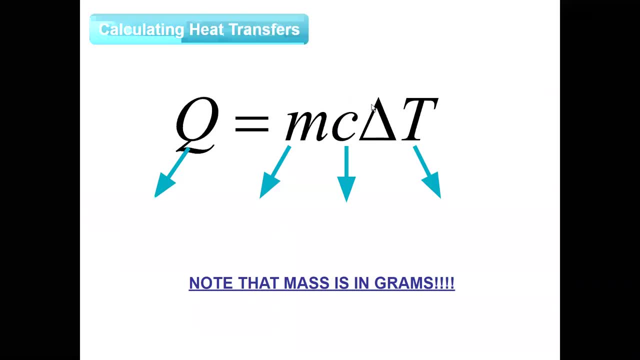 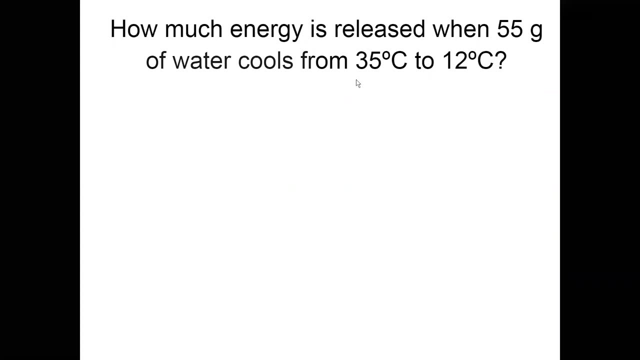 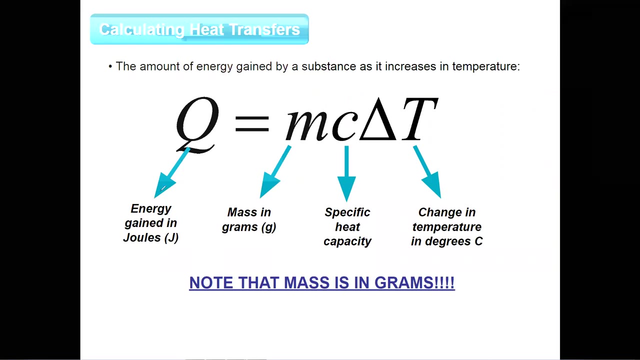 All right, so calculating heat transfers. So this is an equation that represents the amount of heat something gets or loses. okay, So it's a pretty simple formula. Delta Q equals delta MCT, So Q is the energy that you gain in joules. 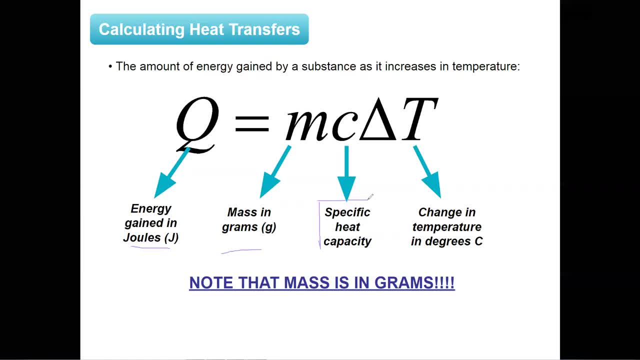 M is your mass, C is your specific heat capacity. So these are all calculated values like observed Observed, So they're usually given on a test. And change of temperature into three Celsius. So change of temperature is the final temperature that you get, minus the initial temperature. 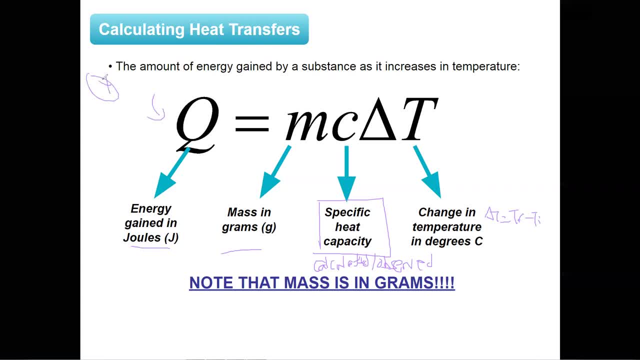 And your value of Q can be positive or negative. So if it was positive, that means it absorbed heat in from the surroundings, And if it was negative, it lost heat to the surroundings. So from the surroundings to the surroundings, And usually what was I going to say? 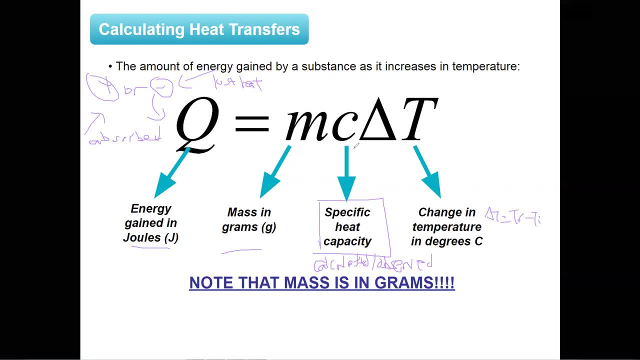 And I always remember this, as Q equals MCAT. But yeah, I believe in science, 10, it is positive or negative, But in chemistry we usually work in positives, although the concept is different. Okay, Okay, Okay. So let's move on to the next one. 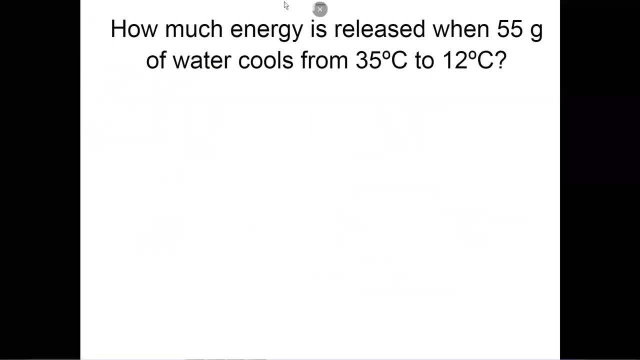 So let me clear all this up, Okay, So let's do a practice question. How much energy is released when 55 grams of water pools from 30 degrees, 35 degrees to 12 degrees Celsius? So this is our equation: Q equals MC, delta T. 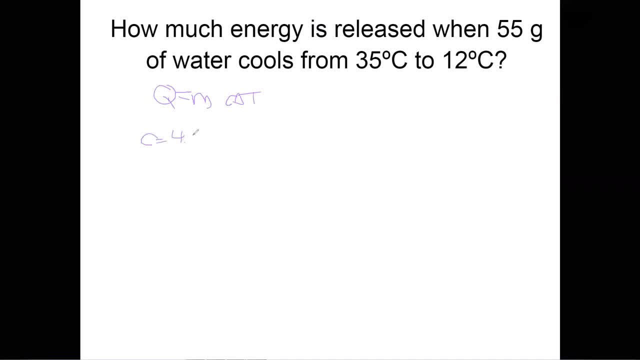 So we know the specific heat capacity of water: 4.19.. joules per gram Celsius. we want the change of temperature, so TF minus TI, we have final temperature. we have initial temperature, so 12 degrees minus 35 degrees, our 23 degrees Celsius, negative 23 degrees Celsius, and then we have the 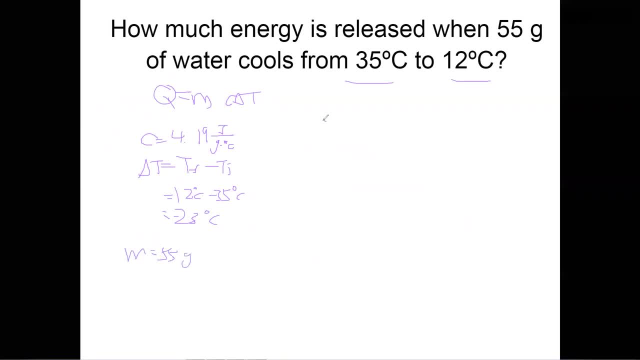 mass 55 grams. so we just simply plug it in. Q equals MC Delta T. Q equals four points. oh sorry, I put it in around five grams here. I know 23 degrees Celsius here, so based on this you can already tell that you'll get an edited value for. 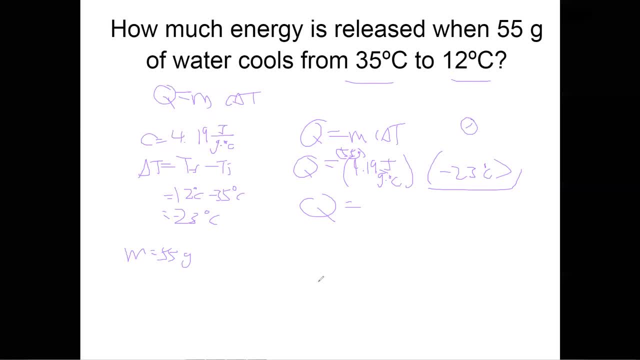 Q. so that makes sense, right? because? because if you're releasing energy, you're losing energy. if you're losing it, your net gain should be negative. so we will just plug these numbers in our calculator, so I have it beside me, let me put it in, all right, and then we get. 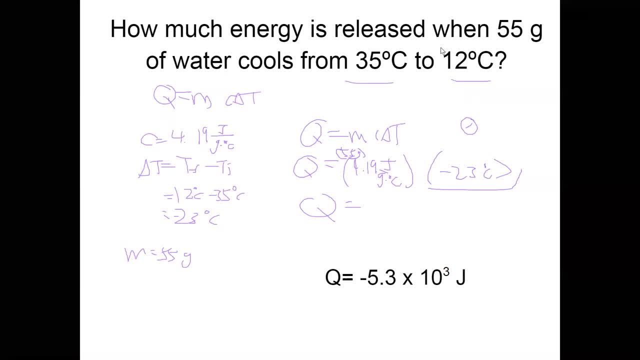 okay, well, very, oh, very interesting. why did I just do that? but um calculator, our raw value is negative. five, three, zero, zero, one point three, five, and indeed we have the round two, three significant digits. so that will be, I mean two significant digits. so there's five point three times 10 to the power of three. 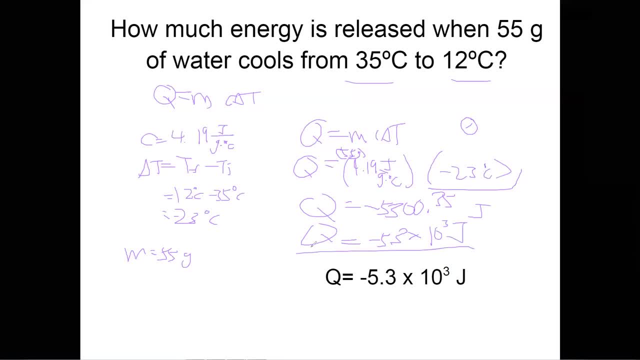 Joules. but you should usually state these questions in a sentence and you're pretty much able to get them in the calculator. I just need to edit these out, but you should usually state these questions in a sentence in the calculator So you would state: the energy released is to pretend that wasn't there not negative times? 10 to the power of three joules. 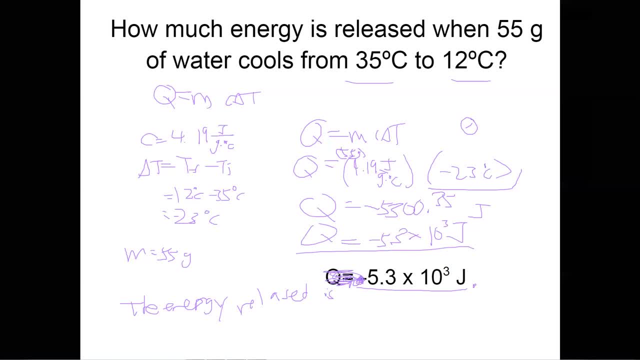 You would just put a positive, you would just say positive. And the reason is because that is just not how you say it, because you are still releasing a magnitude of energy, But by saying it's releasing, we know that the net gain, or the net whatever, is negative. 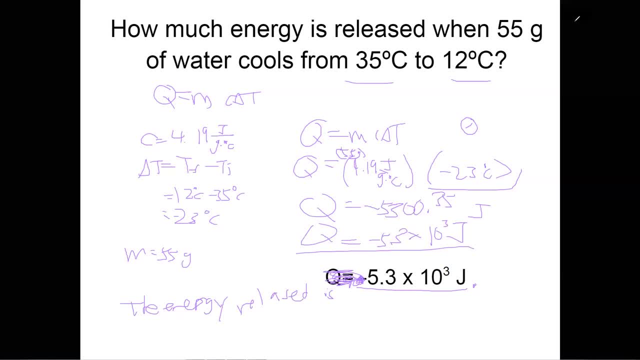 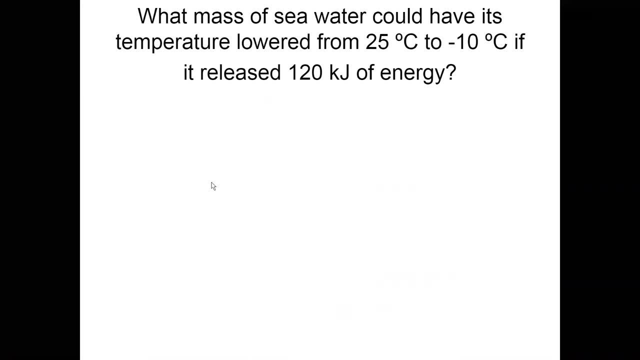 Okay, so let's move on to the next. Okay, so these seven portions are the same, So we'll just go over this. So we'll just say I'll just quickly see how to do it. So 120 kilojoules is your Q value. 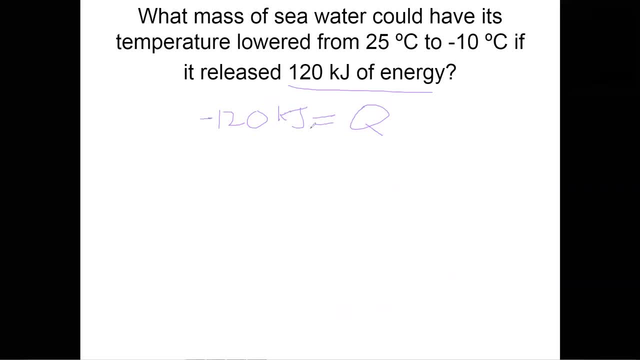 And it's. the temperature is getting smaller, so they should be negative Seawater. We're going to do that. We're going to do that. We're going to assume that it's regular Well, we need the specific heat capacity of saltwater, but I don't have that on me. 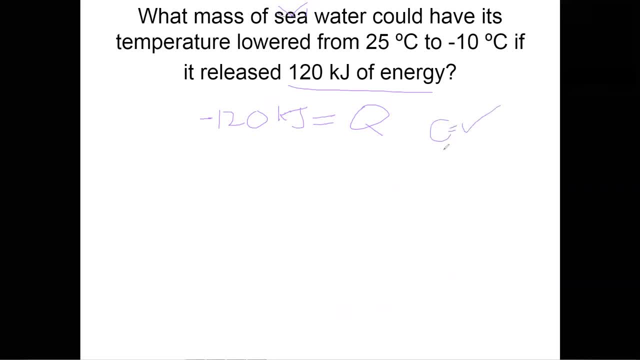 So we'll just say that's water. So you'll know what C is. You'll know what the change of temperature is. You don't know what the mass is. You need to find the mass. Your C value is in joules per gram Celsius, but you want it in kilojoules per gram Celsius. 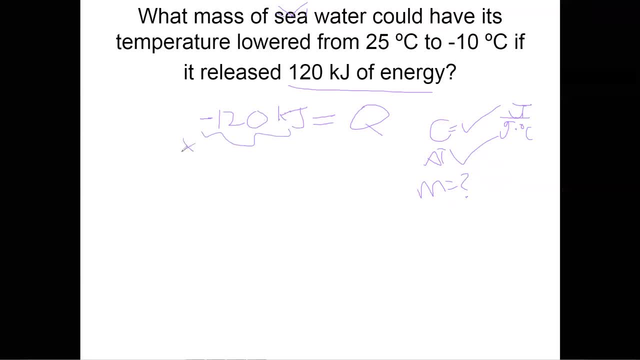 So I would convert this into joules. So to convert from kilojoules to joules, you multiply by a thousand In joules and then now you can use: Q equals MC Delta T. isolate for M. M equals Q C over Delta T. 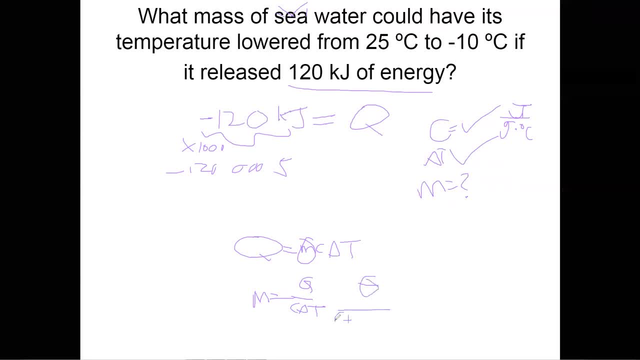 We have a negative Q value, a positive C value and a negative T change of T value that cancels out. So your answer, your mass, will be positive And that made sense because mass is a scalar value. but it also makes sense because we cross it out. 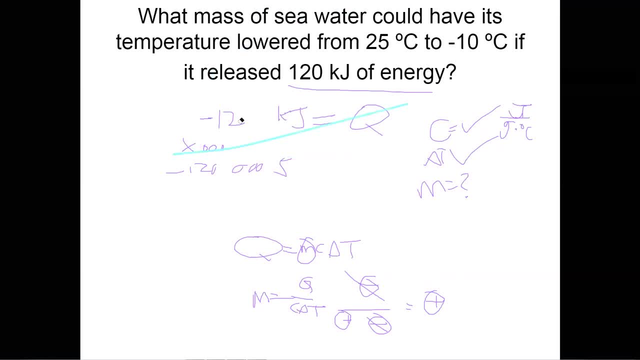 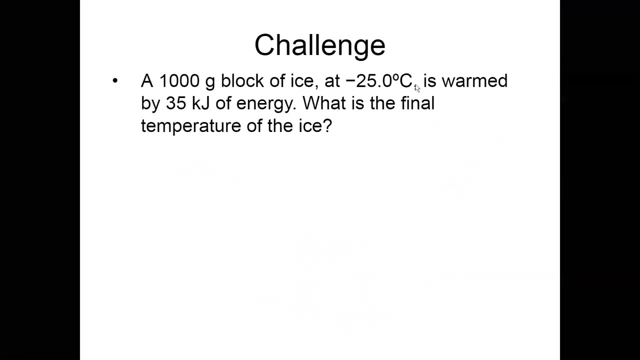 And we induce that. we induce all of these properties of change of temperature and stuff. Okay, let's move on. All right. So this is a challenge question, but we're not doing it. All right. So energy transfer in the hydraulic cycle. 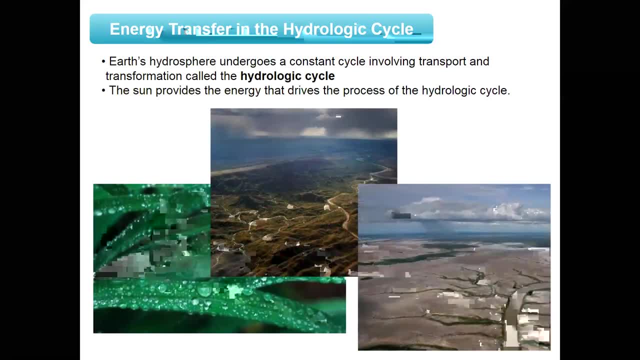 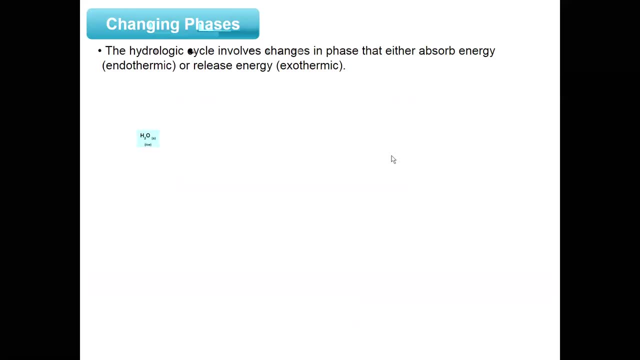 So I believe this is just like the The rain, the rain cycle, the water cycle, right. So in the water cycle, things absorb energy or release energy, right, And things change. So it goes from ice to water, to vapor, which is gas, right. 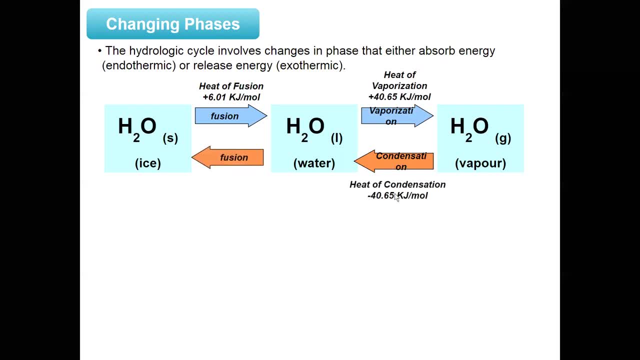 And then there are some certain values of it. So these are the terms essentially, So the terms from ice. so something going from solid to water can be called fusion, something going from Water. I mean, I know I'm sorry, not for something, only for water. 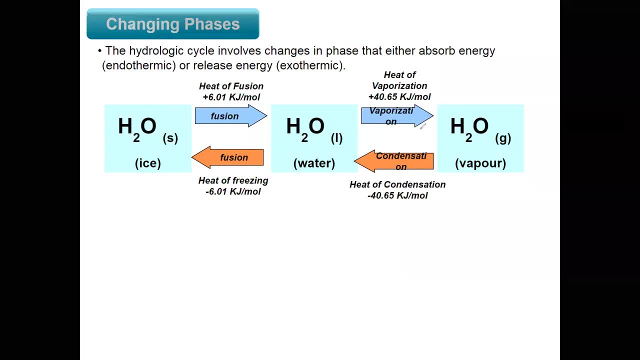 These words apply. So vaporization is from liquid to gas, from gas to water- It's taught in station- And then from From water to solid, it is once again. I mean water to ice. it is also called fusion. 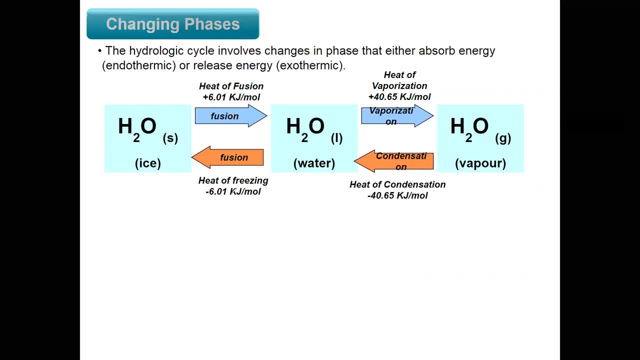 So Two When? Okay, So, if you think about it, So why is one of them positive And why, Why is one the negative? Well, think about it this way: When you heat up water, it starts to boil and turns into gas. 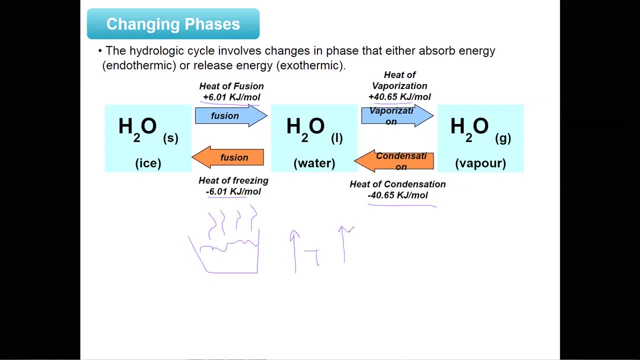 So the more temperature you need, the more energy, the more heat you need. so the more energy you need will make it more of a gas. Okay, so gas solid liquid and the energy increases. The energy applied must be increased as you want to make it into the state. 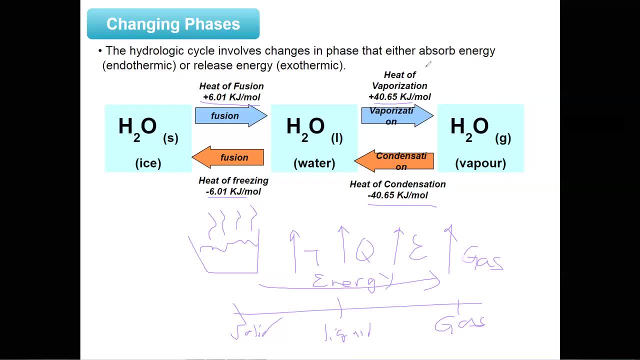 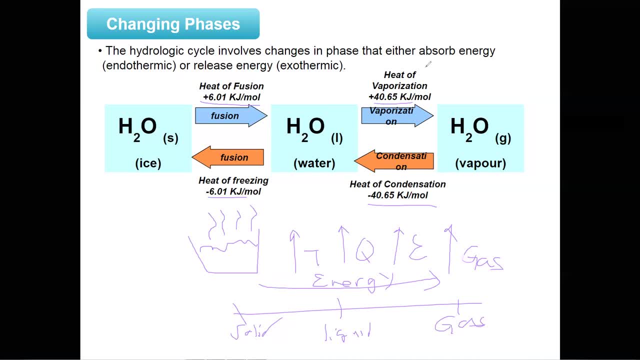 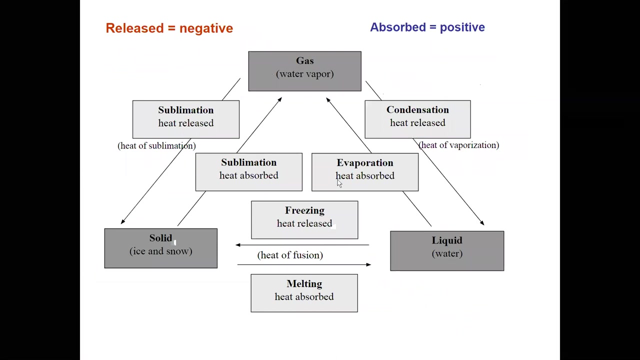 You need to make it more of a gas. You need to apply 6.01 kilojoules to it so that it heats up. Okay, yes, that's it. Okay, let's move on to this one. Okay, so you see all this. 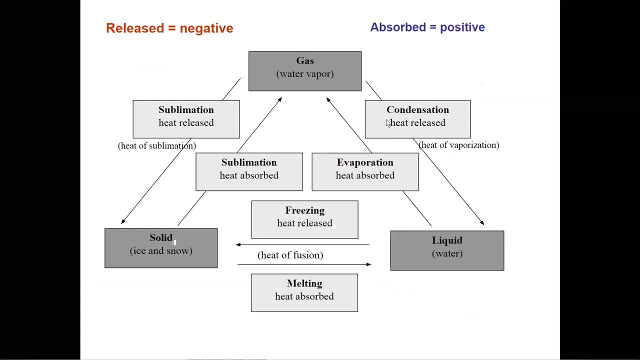 This is just something interesting. Well, this is like. I don't think you memorize it, but it should be pretty easy. Gas, solid liquid, freezing, melting- common terms. condensation, evaporation- common terms, and sublimination is the one from gas to solid. 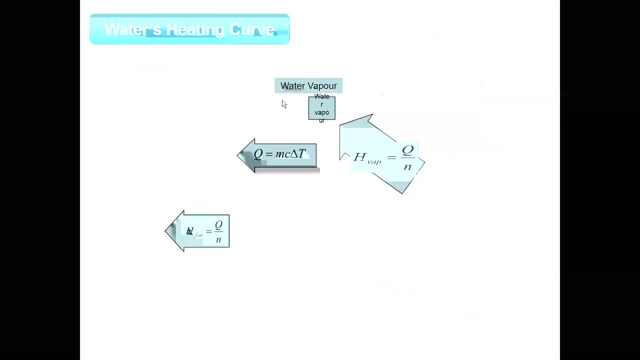 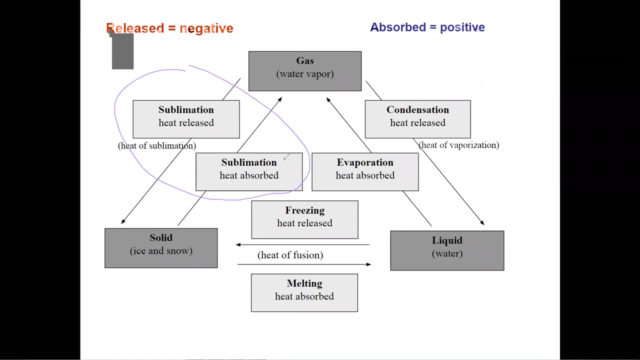 This one is the only interesting one. Wait, sorry, This one is the only interesting one, But it is literally called both the same, So this is actually pretty easy to memorize. These are all common. These are all common. It's just this. but this only has one name. 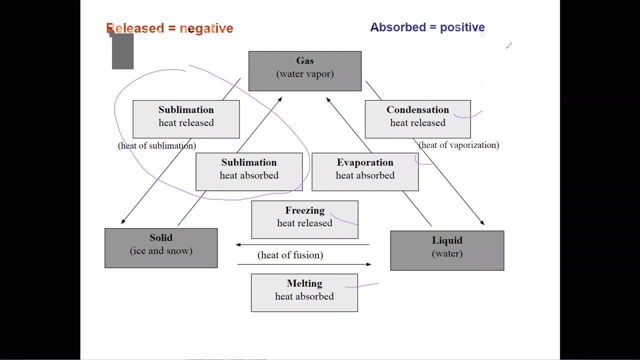 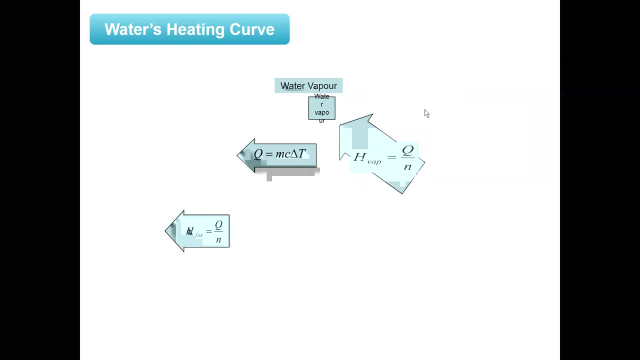 So, from gas to solid, Gas to solid, both ways. it's also sublimination, Okay. So the formula for your heat of vaporization and your heat of fusion is you take, Is that you take? Is that you take the amount? 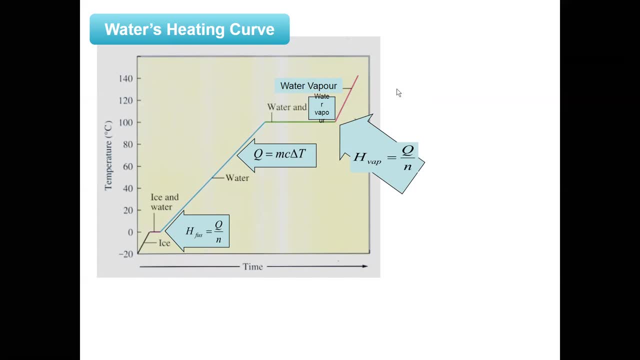 Is that you take the amount of heat absorbed or lost and you divide it by the amount, The amount of moles- you have to find the heat of fusion and heat of evaporation. See the amount of heat it takes to make one mole of water or ice. 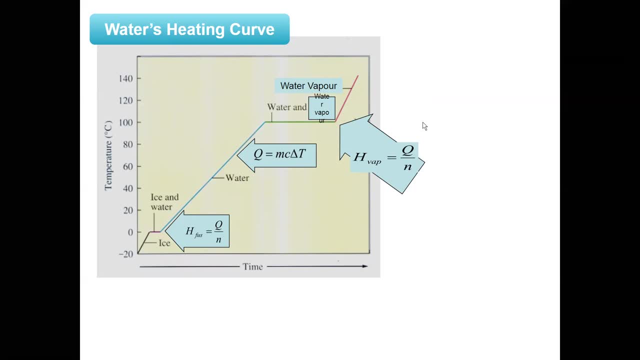 Of ice turned to water or water turned to ice. Okay, That is what it basically is saying. So a key note is that when the state of your water is changing, when the state is changing, so your temperature does not change, And vice versa. 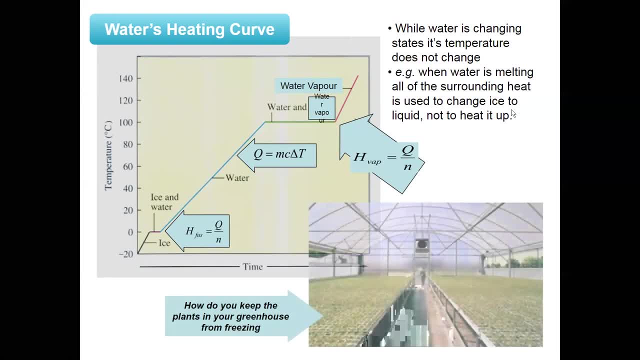 So when your temperature is changing, your state does not change, Right? So when water is turning into ice, it changes at a certain temperature, which is your degrees, Right? But the but the temperature remains constant. But when you are changing the temperature of something, 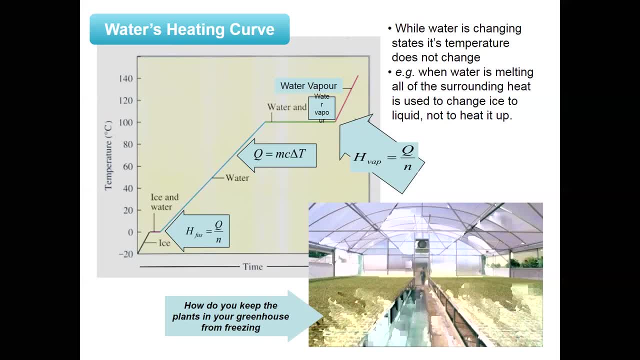 the state of it does not actually change. Okay, So let's make sure the temperature changes. That means Let me change the temperature of my cell, And that is where the temperature changes. So I don't care how much I change the temperature in my system. 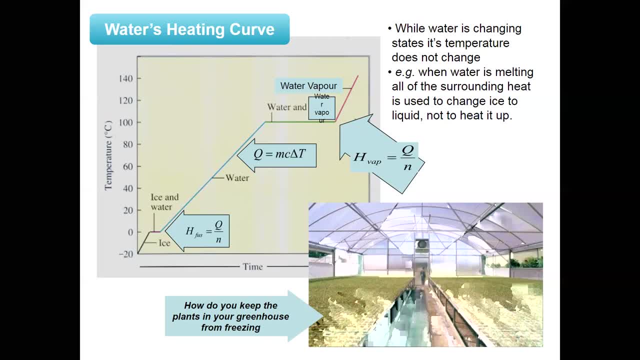 The temperature changes her temperature. When the temperature changes, I am always changing the temperature And it is slowly because I don't want to wait 10.. I have already changed temperature, Okay. that means 10 exact times, Okay. 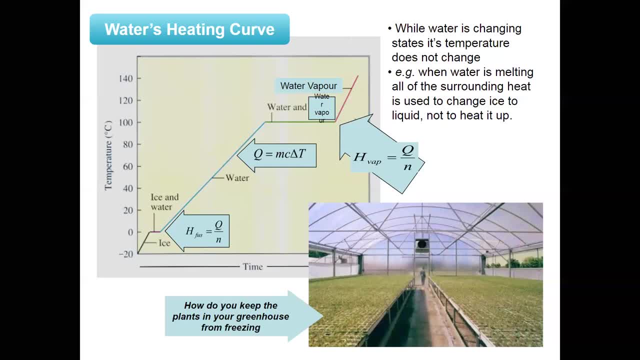 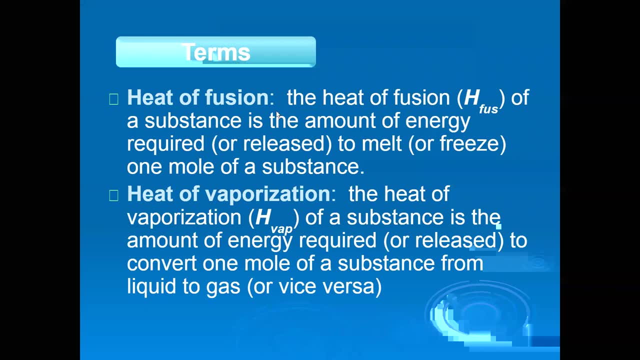 Ok, next question is what I was talking about We. how long does it take it? You are still in small regions. You and I have many businesses in small regions. How do you manage it? I feel sorry for that. heat of fusion, substance of energy required to release or melt, freeze one mole of a substance. 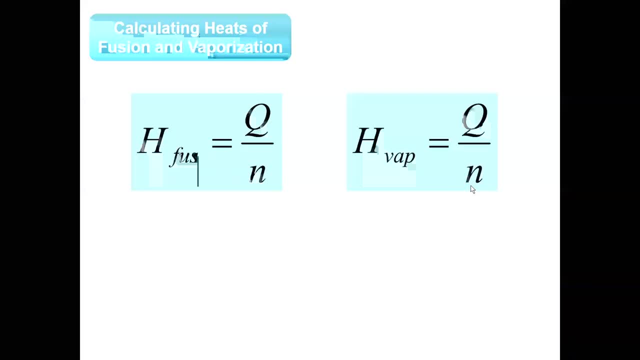 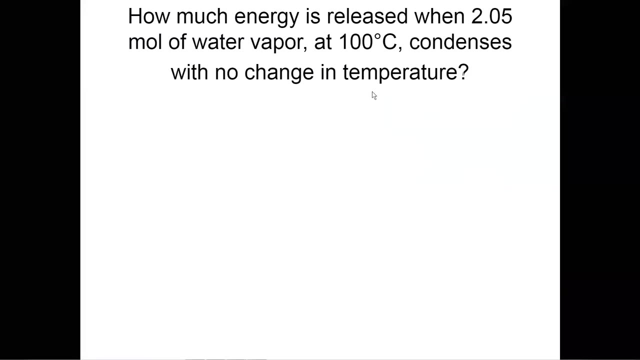 vaporization is just vaporize a substance. so yeah, so q over n. we went over how to do this okay, so let's see these questions. so we know. the formula is: h equals q over n. how much energy is released when 2.05 moles of water vapor condenses at 103 celsius with no change in room? 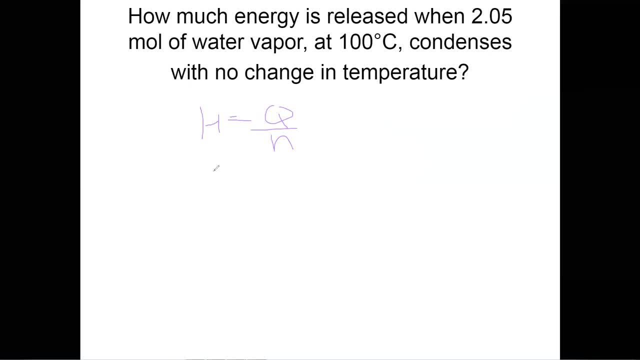 temperature. okay, um, you isolate for q n times h and you know your h value. your heat of vaporization is 40.65 maybe. so i will just multiply 2.05. so i will just multiply 2.05 moles times 40.65 kilojoules per mole and i should get the answer. 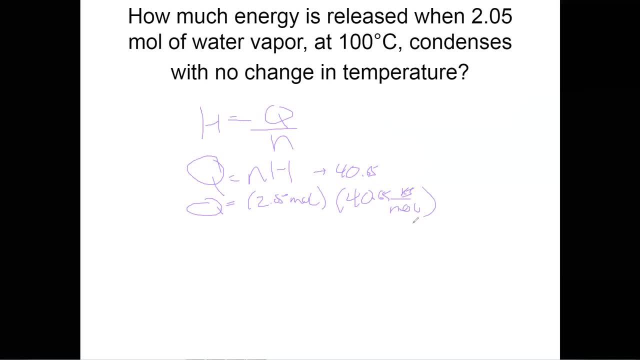 all right, so i got 83.3. so choosing it once in the three significant digits is 83.3. so let's go see this. oh, okay, and it's negative because, um, i should have added the sign sorry. and it's negative because water vapor condenses, so it goes from gas to liquid and we just demonstrated that from. 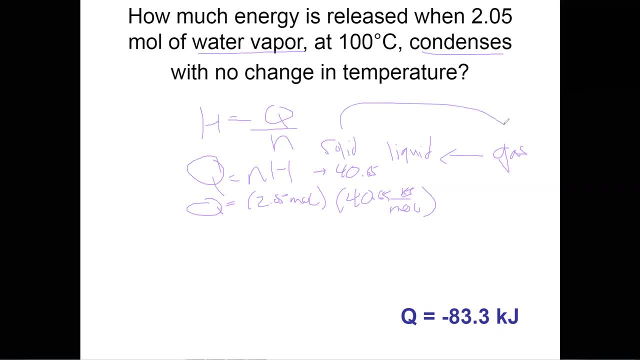 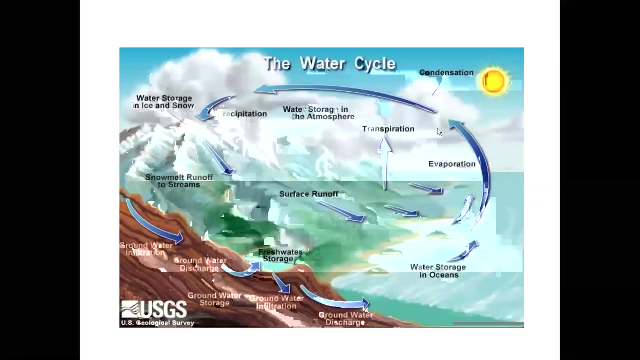 from solid to gas, you need to add energy, so that means from gas to liquid, you do the opposite, so that means you release energy. so it should be negative. and this would be- and this negative would come from the h value- negative. okay, all right, and we know all this. okay, so let's just read over the water cycle. 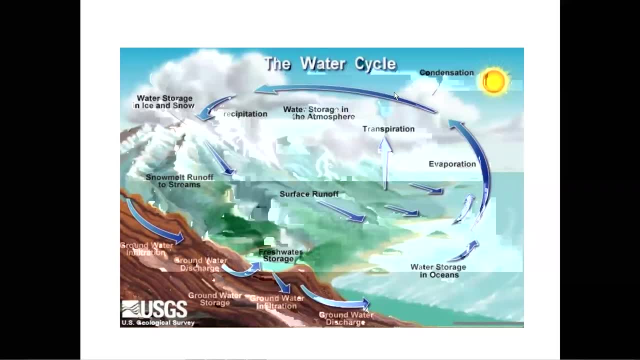 evaporation. water is drawn up from, drawn up into the clouds, from the heat of the sun inside the clouds it condenses into water. the water falls down and it's called condensation. and then the heat of the sun goes up into the clouds, so it condenses into water. and then the heat of the sun goes up into the water, so it goes up into. 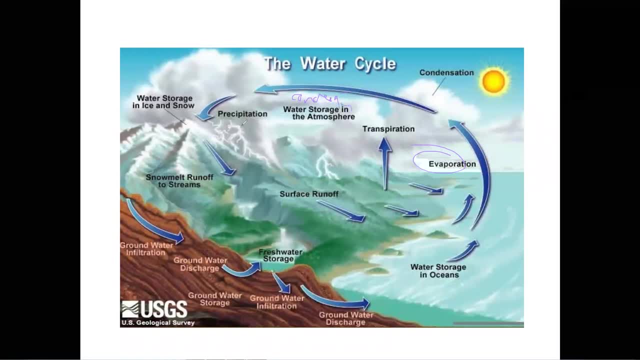 the third step is precipitation. so one, two, three, yep, that's it and all these things. it's basically saying: um, well, water and plants and from the earth is goes up by transpiration, and the runoff just means that when it hits the earth, it may flow and collect into like something else. 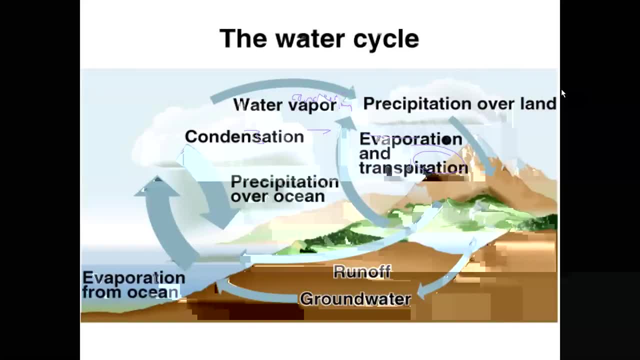 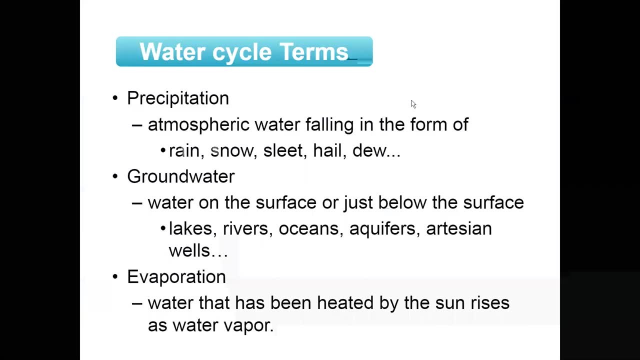 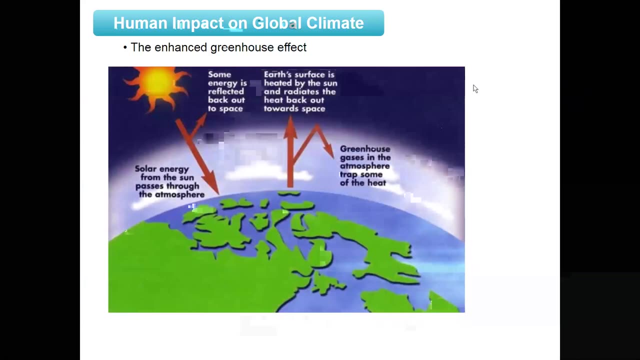 okay, um, yes, this is the water cycle again. okay, let me erase my drawings, so i was going over that. okay, easy. so human impact on global climate. so greenhouse effect. we emit greenhouse gases into the atmosphere and some of the major ones are co2. you probably heard that co2 is really bad because it traps in the heat molecules and 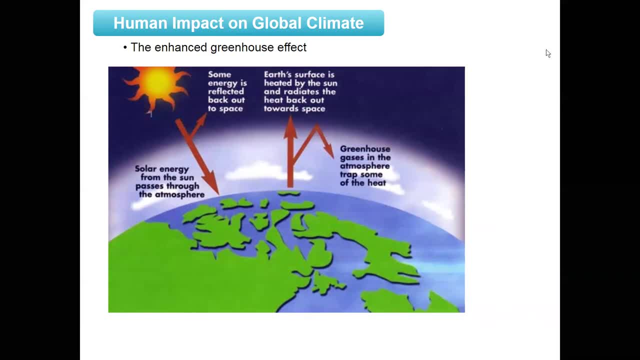 we do the, we do the, we do the. a lot of our tasks, like, like driving and using electricity does, um, does, promote more co2 in factories. so basically, uh, human impact is that because of our desire to have things that we don't necessarily need, like factory items and cars and luxuries- 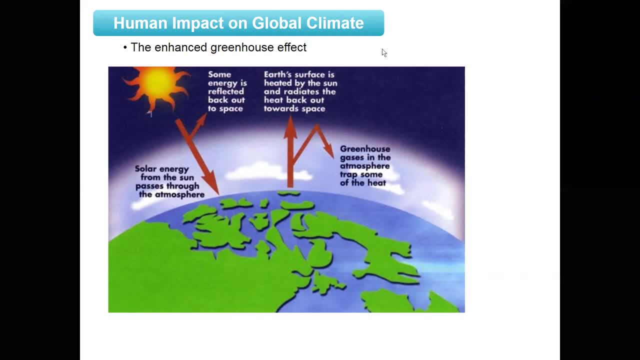 we are actually damaging ourselves in future generations because, oh, there's something in chat. hold on, i did not, i did not, i cannot tip the chat um, let me just ims you this, but uh, yes, that is what human impact is. yeah, so co2, ch4 and 20 h20 water vapor. 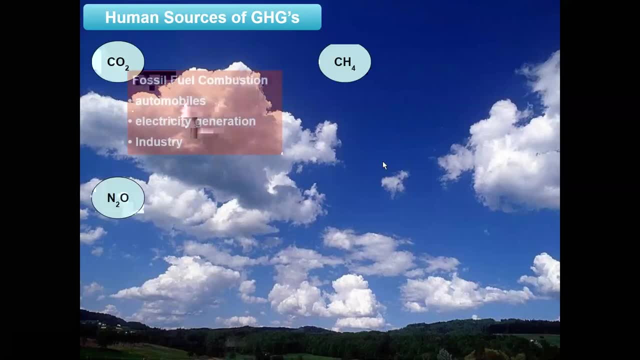 all right. so, yeah, industry and electricity, automobiles. that's my co2 example, the tail with the austria percent livestock. yes, cows, they, they poop a lot. so that's why they produce ch4 n20. i believe it's from. like cars. yeah, cars and fertilizer okay. 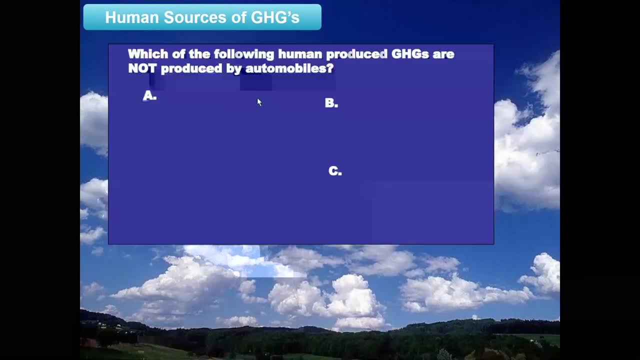 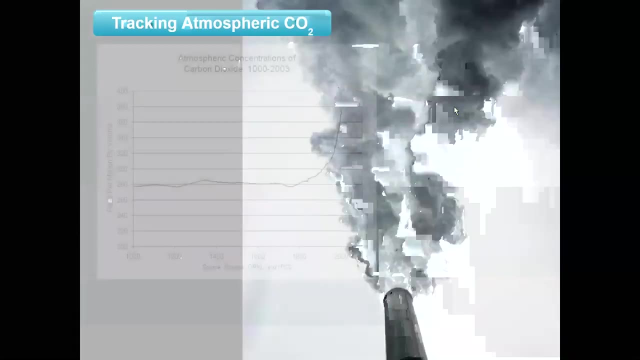 all right. which of the gags are not produced by automobile co2 and 20 or ch4? it is ch4 because they are only made by cows and other things like that. all right, so how do we track co2? well, um, i'm pretty sure you measure like ice. yes, you do so. 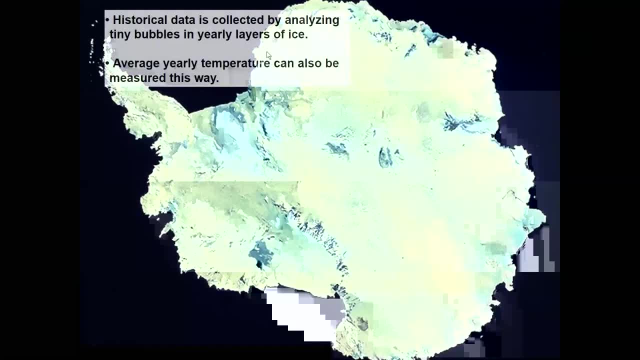 you look at ice and things that have co2 trapped in them from years ago and you can see it compared to the average co2 concentrations and other things, like the ice today compared to the ice sheets found millions of years ago, and we do see an increase of co2 which can kind of be attributed to the high amount of evidence that. 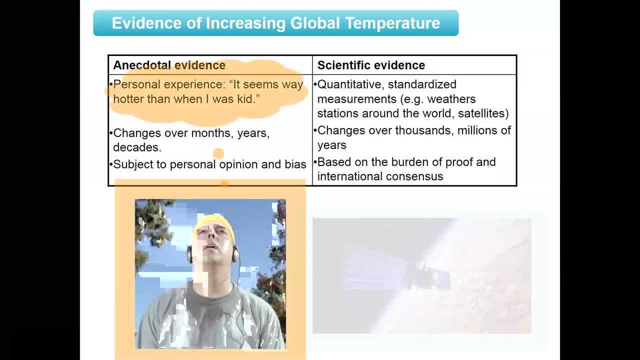 we get, and that is what is currently being done, because the reason why this has happened so far is that because of the average co2 concentration of over 30 million tons of carbon dioxide, which is probably about half of the average co2jugations that have been produced today by舒in. 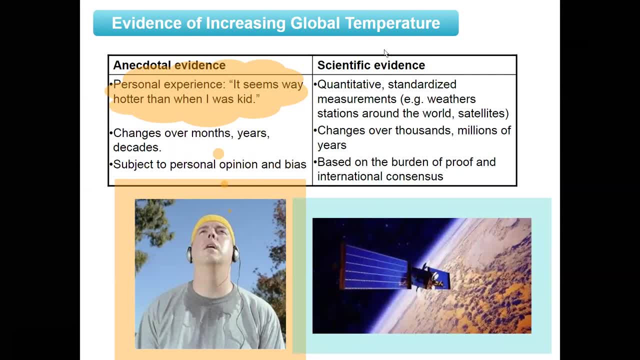 kind of support which does support that the earth, climate change, is real, unlike these hate, unlike these fake people saying that it's not happening. so just some quick terms, anecdotal evidence: these are stories, these are things that you come up with yourself. it's not really evidence. 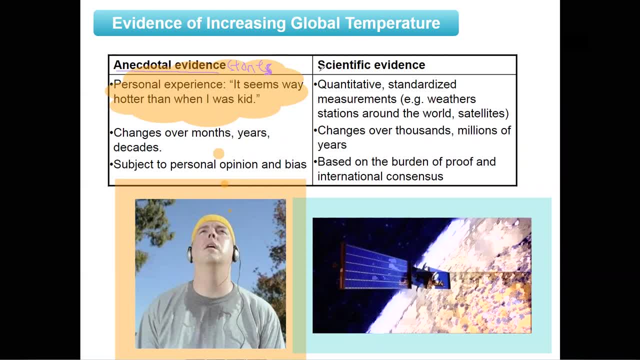 because you have no recorded proof of it. you're just saying it based off memory, scientific evidence. it's evidence. there's like um, um, it's like hard evidence. it's like i forgot what the word is, but it's just. there's just there's evidence to. there's proof, right, and you go through multiple scientific 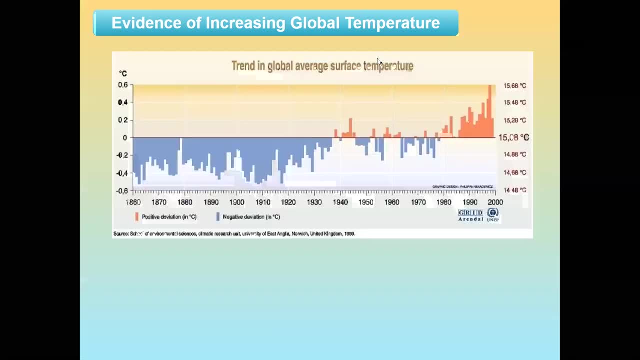 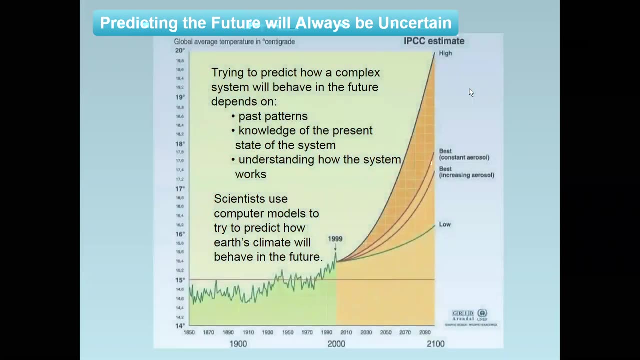 processes to verify that your data is accurate. all right, so the temperature is changing. all right, so, uh, all these things are just saying that science. scientists should track our future by looking at various data such as carbon dating, and they can predict how bad the weather is going to be, and it is pretty bad because they predicted that at the 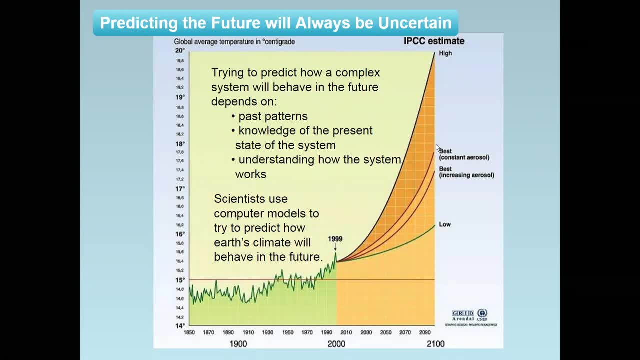 end of 20 to 100. so 20, okay. so 2000 and 2100. uh, we cannot reverse climate change anymore and it will increase by one degree, i think. from now to 20, 20, 2100. it increases by one degree, which may not seem like a lot, but after that it will. 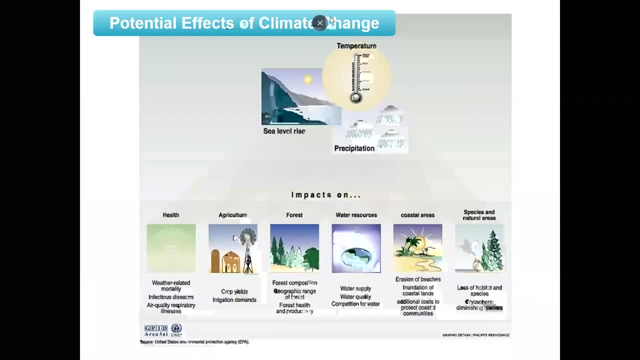 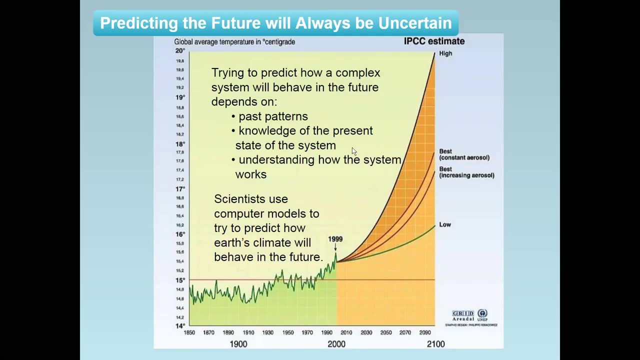 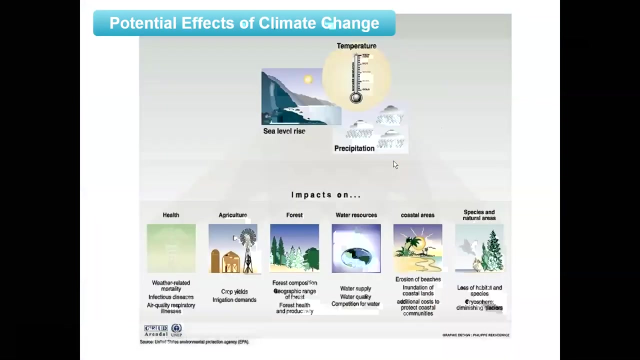 actually that presenting like that graph is pretty old. the new prediction is that world's gonna essentially end at like 2050s. so have fun, guys. actually, yeah, oh, oh, yeah, it is pretty old. oh, it is really old, isn't it? wow, so we might end, but that's not my issue, that's their issue. 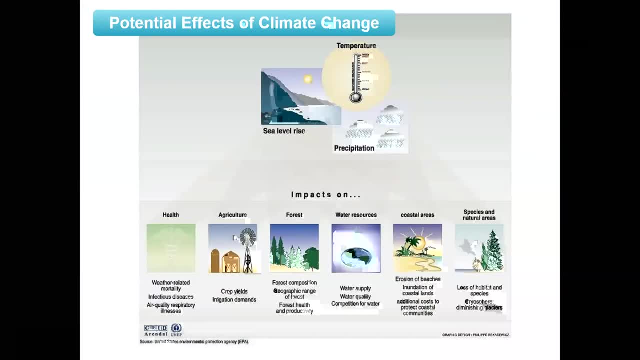 so what are the effects? well, obviously, climate change will make things harder and the sea level will rise. never i forgot why the sea level rises, but anyways, the sea level will rise, right and and the sea level rises. homes are destroyed, crops they ran out, animals lives cannot animal lives. 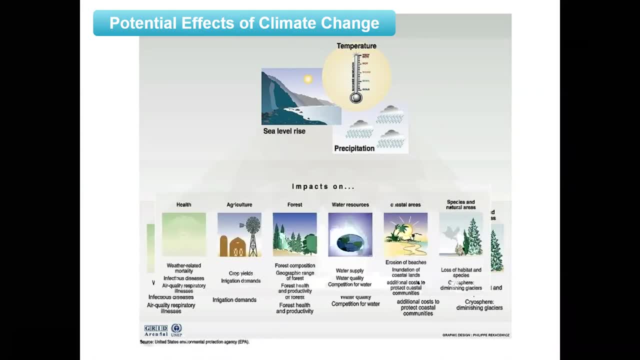 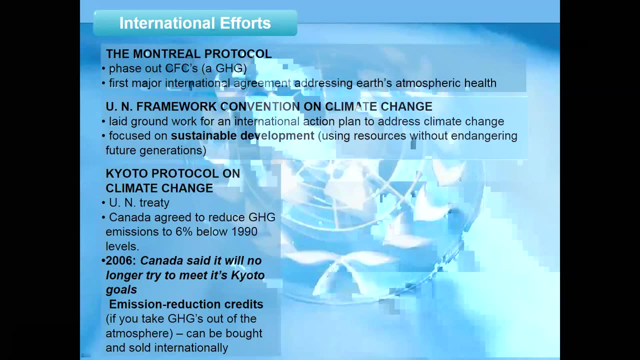 cannot be sustained and all these things, okay. so international efforts: you don't even know these at all, but we're just gonna put them here. montreal, un, toyota protocol- um, i think you learn about toyota protocol and social. that's not important as well. socials are not important in general to 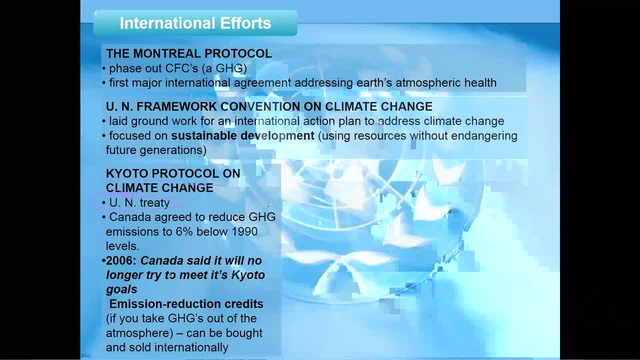 be honest, but, um, un, i don't know. um, that is, i would say. the main thing. takeaway is that we are trying to make efforts to stop climate change, but obviously the national interests of nations today it is to it's other things like they, they like their economy, they like government, they like. 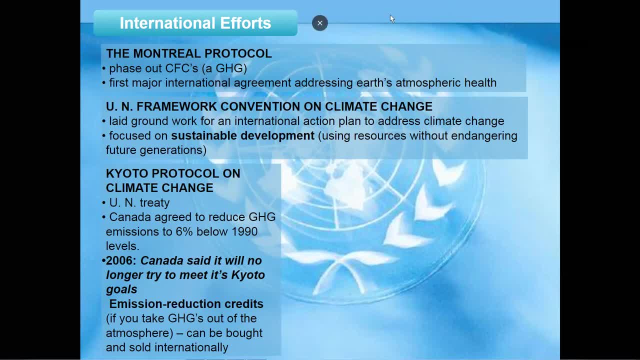 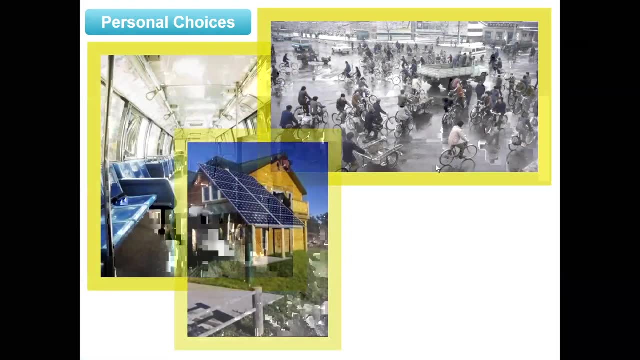 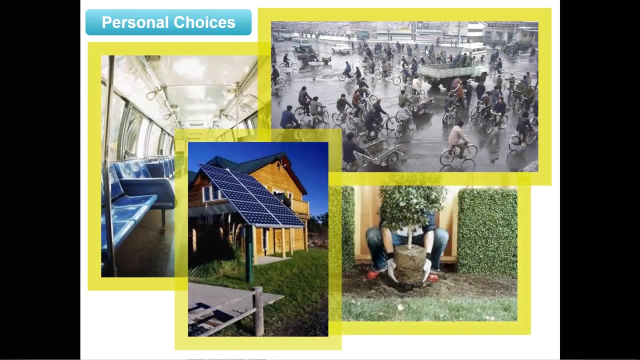 political affairs, foreign policy, they like all these things over the environment, so don't expect much, please. all right, and this is just personal choices. uh, you can reduce your impact on climate change by well planting trees. not really, but like sure, every little step counts if we all. 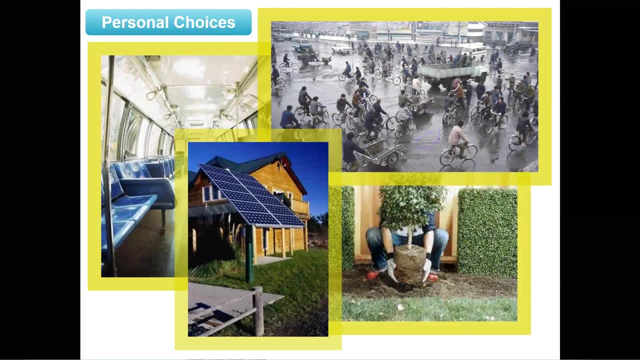 work together. so you see how these people are invites. they are not amazing. ch4 and co2, i mean. uh, not co2. uh, they are not in a not co2ch where they are not emigrant co2 and n2o. so, uh, this will help reduce greenhouse gases. they are not using that much electricity. they're not. 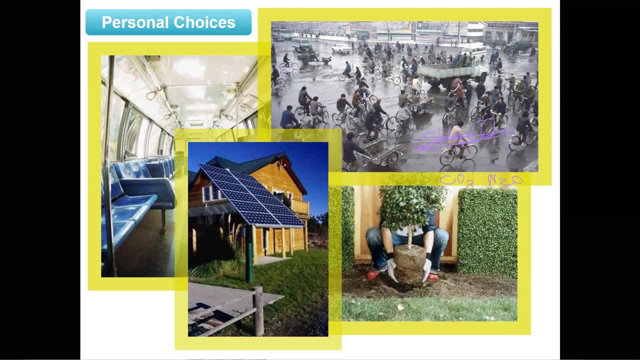 using water and resources, so they are also helping global warming. and they are planting. these folks are planting trees to reduce carbon dioxide levels because photosynthesis plants need carbon dioxide, so this is also helping. so you can make. so. the main moral is: the environment is not environmentally conscious. use a hydro flask and I believe that is the end of 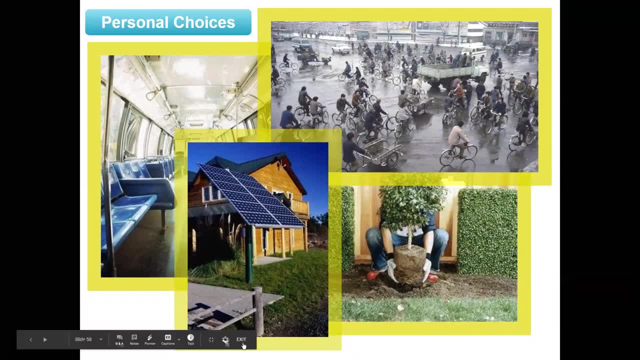 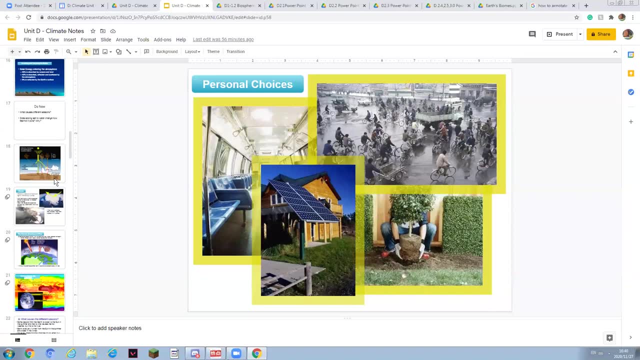 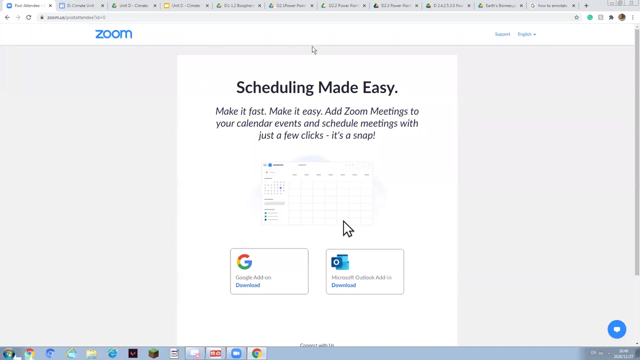 global systems. yes, slide 58. so, with that in mind, that is it. that is science. 10 in a nutshell, in a very large nutshell, but it was a fun experience to teach and it was, and I feel like it was, learning experience. you know highs and lows, but 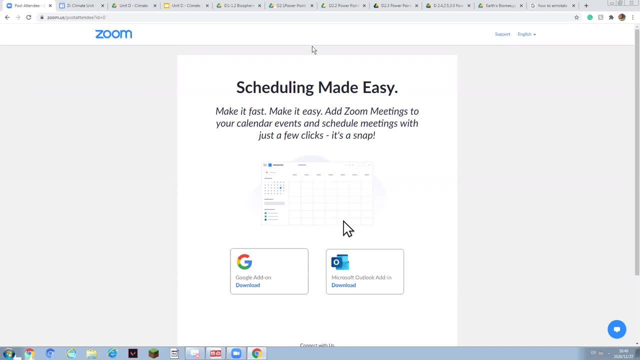 overall, yeah, it was not bad, but if we did make your learning experience harder than easier, I'll apologize, but it is. it is. I feel like we did it a lot harder than normal. if we had a chance to do it a little bit, more did a simplification of everything, so don't stress guys. okay, uh, do you have any closing remarks to?